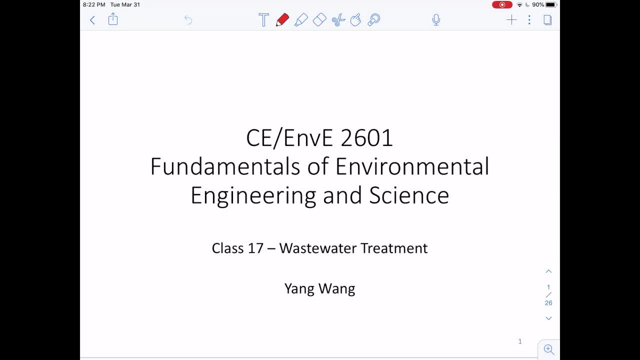 pretty good. So, starting from this class, we're going to learn about the wastewater treatment. So if we go back or do a recap of our last section. so basically we talk about two chapters. The first chapter is about the wastewater treatment. The second chapter is about 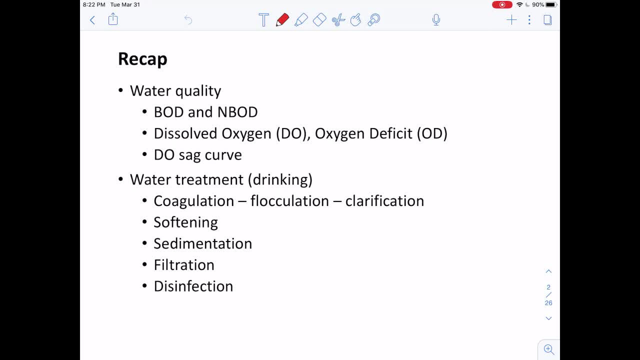 the wastewater treatment. So if we go back or do a recap of our last section, so basically we talk about two chapters. So if we go back or do a recap of our last section, so basically we talk about two chapters Or two types of contents, right? So we talked about the water quality, and water quality was. 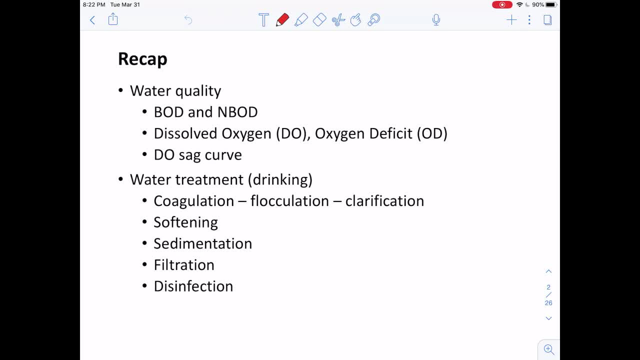 specifically mentioned about the new idea or new concept, which is the biochemical oxygen demand, which is the oxygen that's demanded by the microorganism in the water to oxidize all of the organic components. So also mentioned about the NBOD, which is the nitrogenous BOD We mentioned. 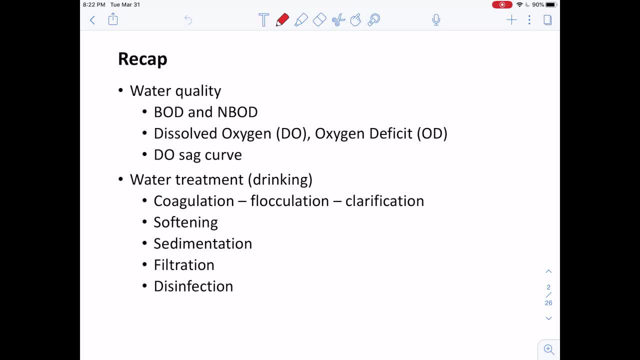 about the concepts for the dissolved oxygen, which is DO, Oxygen Deficit, and we use the oxygen deficit or the OD to solve for the DO-STAG curve right And further in terms of the water treatment, although we did not specifically mention about this definition. so basically, for the water, 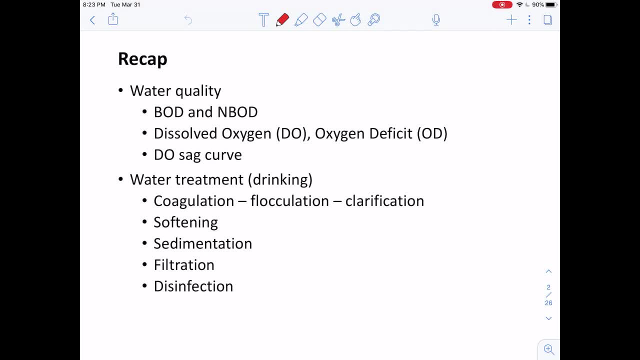 treatment. we're trying to deal with the drinking water treatment system and starting from this. So in this class here we're going to talk about the wastewater treatment. So for the drinking water treatment, we learned about the basic processes such as the coagulation, flocculation and clarification. 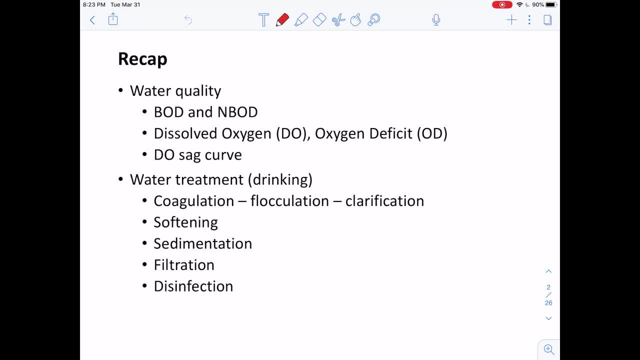 We talked about the softening, which is mainly dealing with the hardness of the water, And then we learned about the sedimentation, which is using the gravity of the suspended particles or the heavy particles to remove those contaminants in the water. We learned about the filtration and also the disinfection at the end. 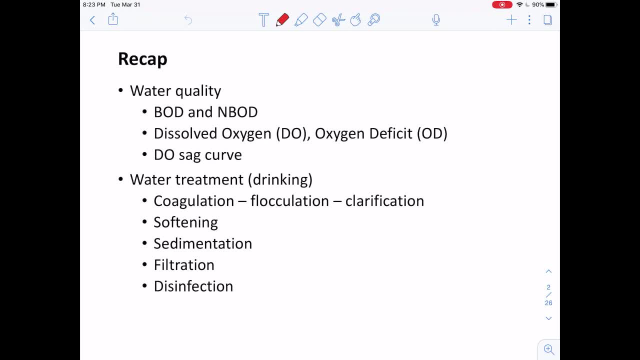 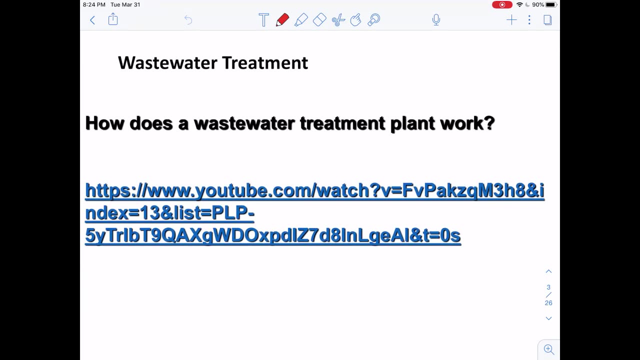 So, as you can see later from this third section of the course, here you can see that we are going to use some similar devices to purify the wastewater. All right, So Why do we care about the wastewater? We know that the drinking water is vital for the human being because we all need clean water to sustain ourselves. 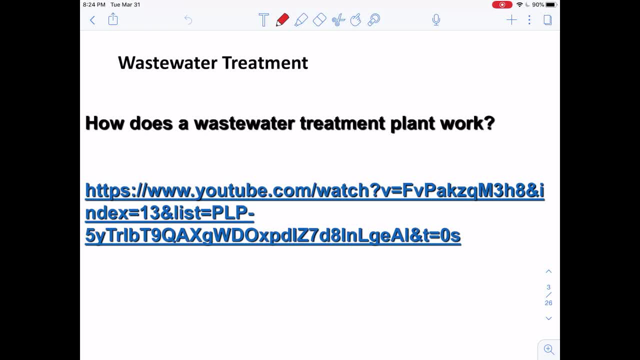 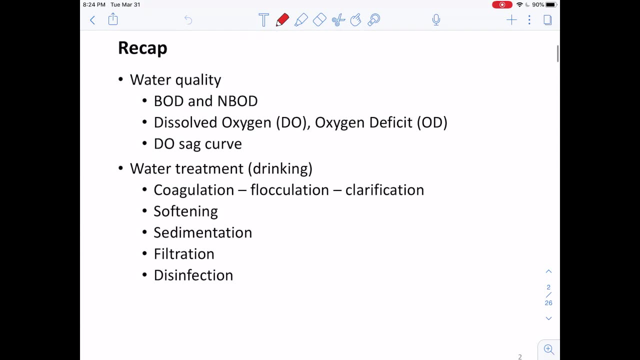 But why don't we just dump all of those wastewater back into nature? Doesn't the nature have its capability to accommodate this wastewater? Actually, it's not. So during the process, when we were trying to learn about the deal sag curve, here we actually find out that when the BOD of the sewage water is higher, above certain value. there the dissolved oxygen might get to the critical point where the dissolved oxygen concentration dropped to zero, And that's going to exterminate or remove all of the living organisms in the water, which is a disaster in terms of the water quality. 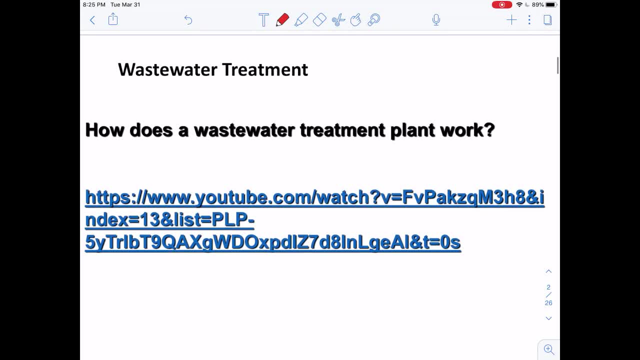 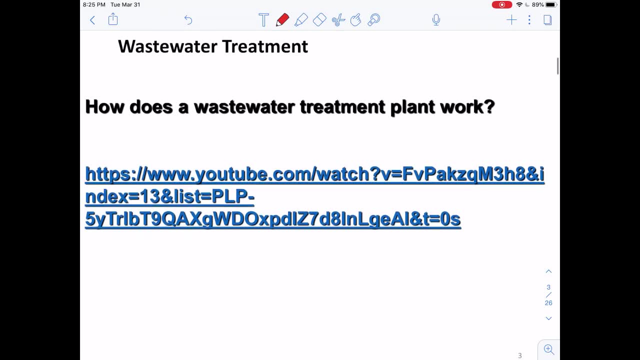 Right. So that's why we have to treat the quality of all of these wastewater before we dump them back into nature. So here I have a short video which is talking about how the wastewater treatment plant works. OK, so let's all go through it here. 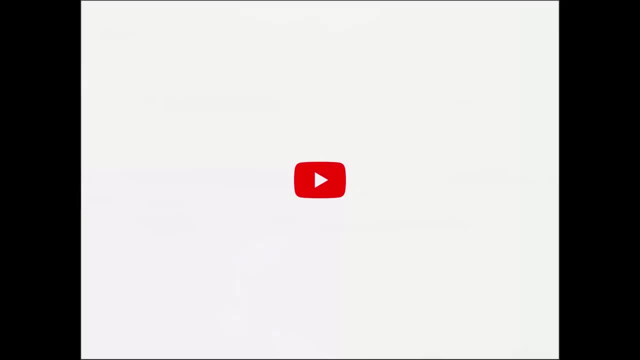 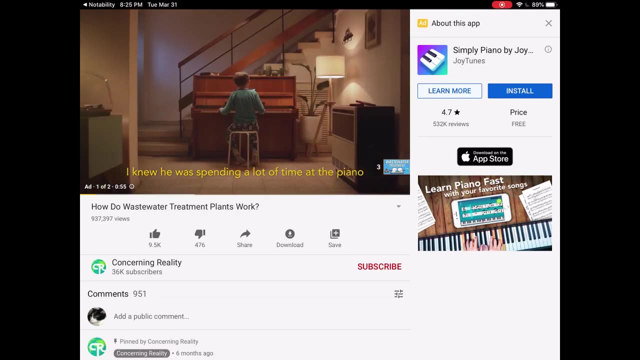 I knew he was spending a lot of time at the piano, but I was doubtful he could get that far. I knew he was spending a lot of time at the piano, but I was doubtful he could get that far. It's a topic we'd rather not think about. 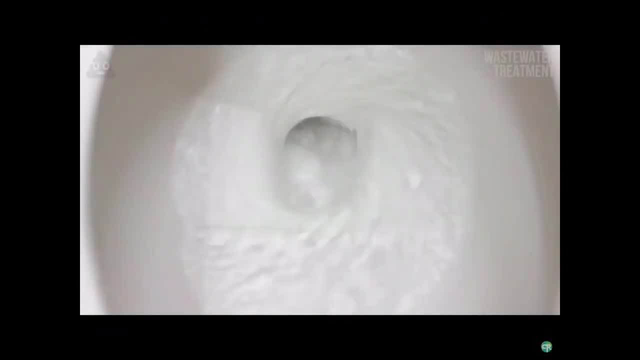 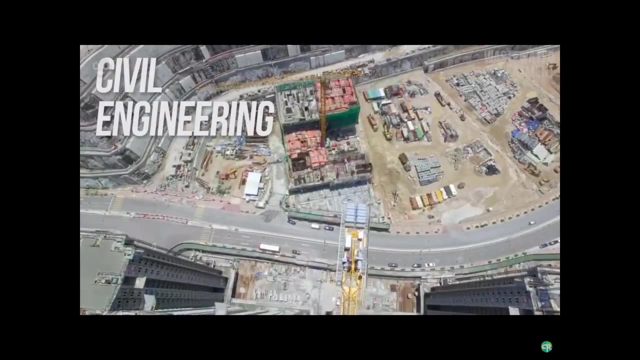 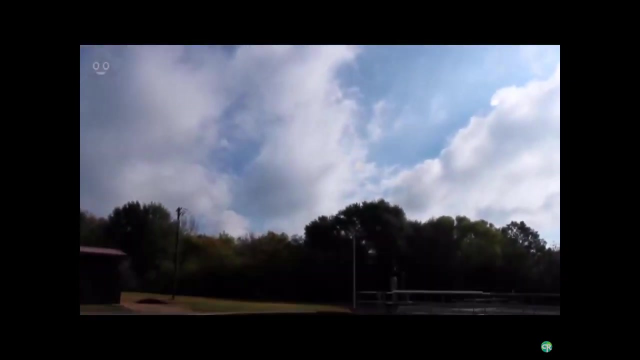 Where does last night's dinner go? Well, you may already be grossed out just thinking about it. This question leads way to a significant subset of civil engineering and a massive amount of public funding. Just like all dogs turn back into water, all drains in a city lead to a wastewater treatment plant, where that wastewater gets turned back into water that we can drink. 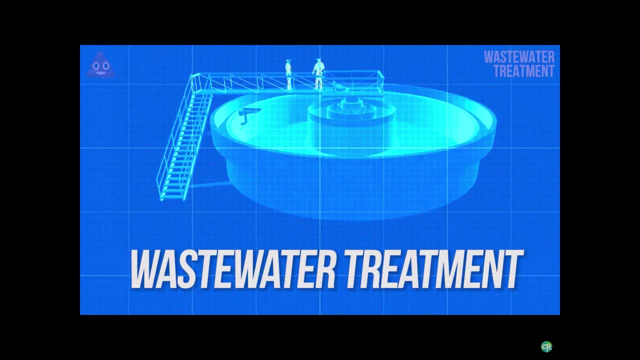 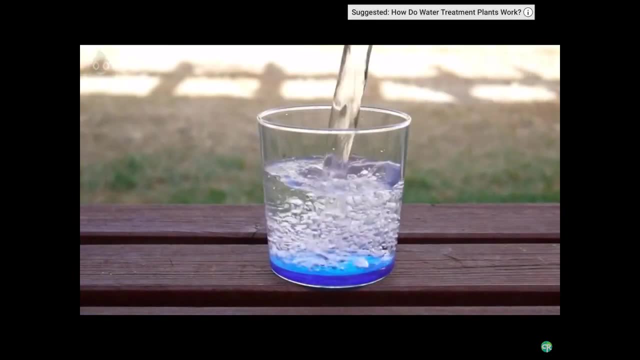 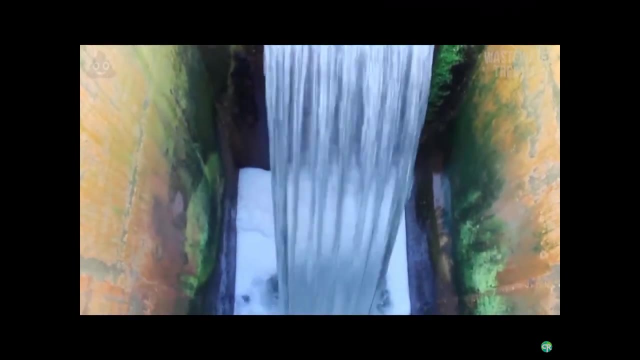 Now you may be thinking that you'd rather just let bygones be bygones and not think about this nasty part of our life, But here's the thing. Chances are, you drank water that was waste at some point, So you might want to take some time to understand this engineering process that makes dirty water clean. 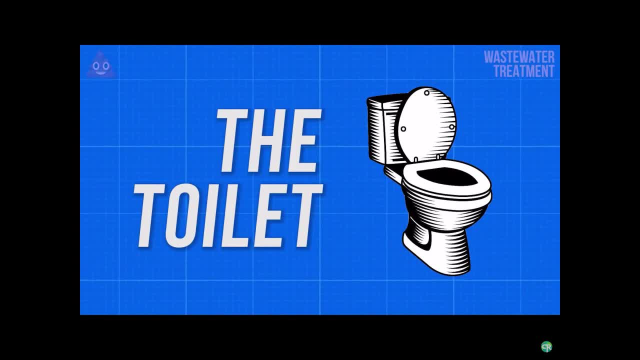 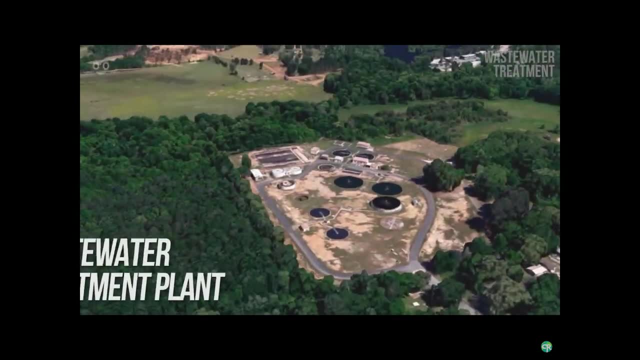 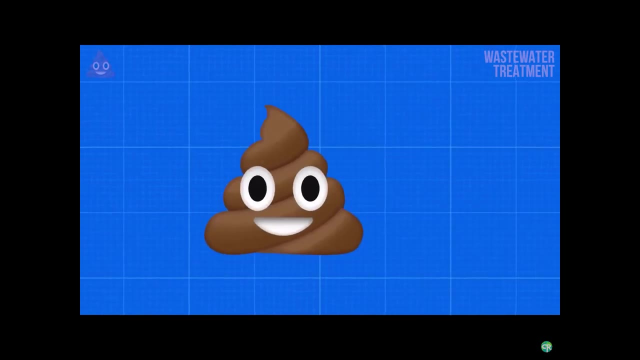 Here's where it starts, The toilet. Once you're done doing your business and flush that magical handle, your waste ends up at the inlet of one pretty interesting place, A wastewater treatment plant. Why is this place so interesting? Because it takes arguably one of the most disgusting substances in the world and turns it back into something that is essential to all life. 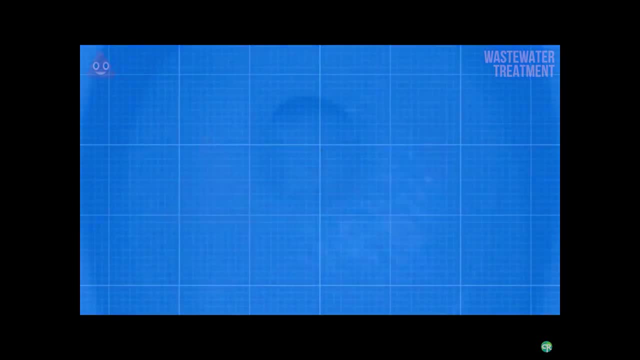 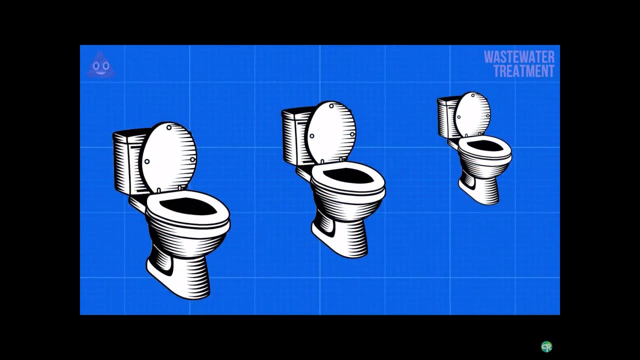 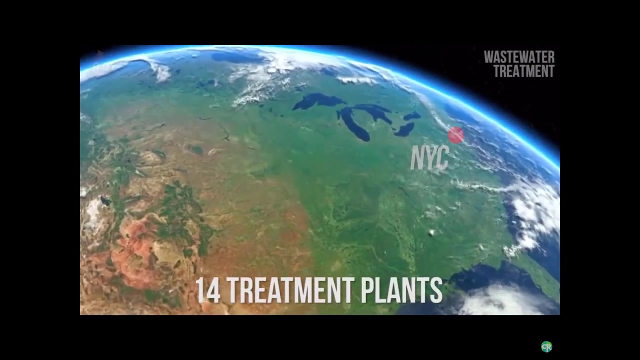 Flushing just your toes and others doing the same thing can result in some pretty high sewage flow rates. If not millions of others doing the same, it can result in some pretty high sewage flow rates. New York City has an array of 14 wastewater treatment plants that handle a combined 1.3 billion gallons of wastewater daily. 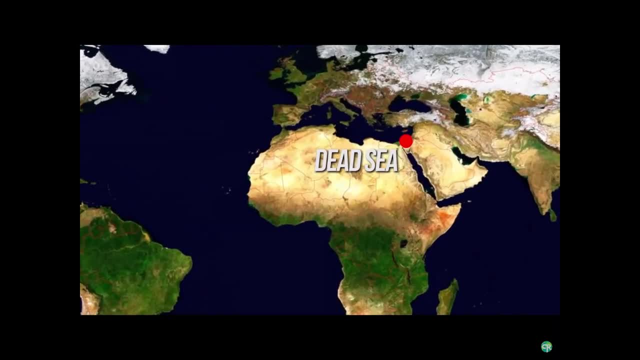 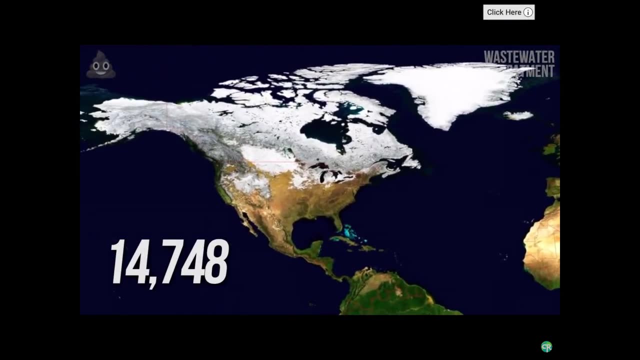 That's just New York City. There are an estimated 14,748 treatment plants in the US alone, And that's just New York City. There are an estimated 14,748 treatment plants in the US alone, And that's 76%. 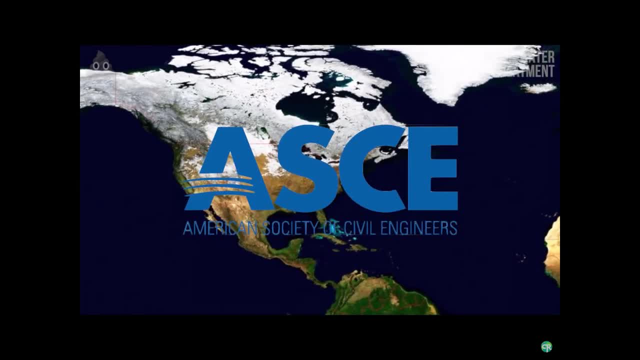 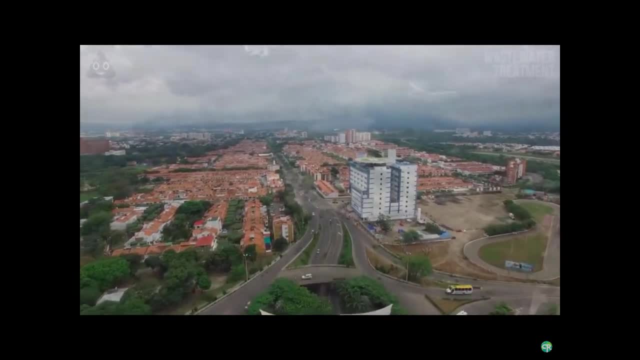 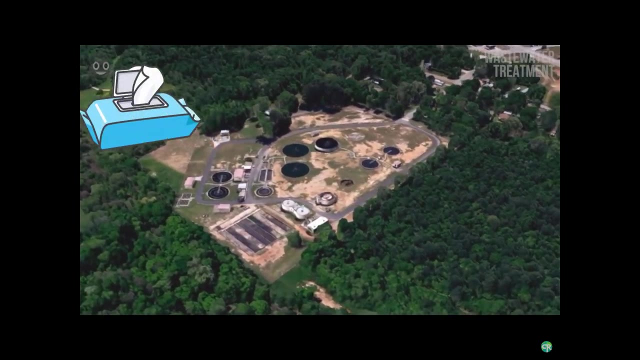 The US waste population relies on warning to the American Society of Civil Engineers. Understanding wastewater is crucial to understanding the critical infrastructure needed to support modern life. That brings us to the first step of the process that handles toys or even guns, Things like flushable wipes. 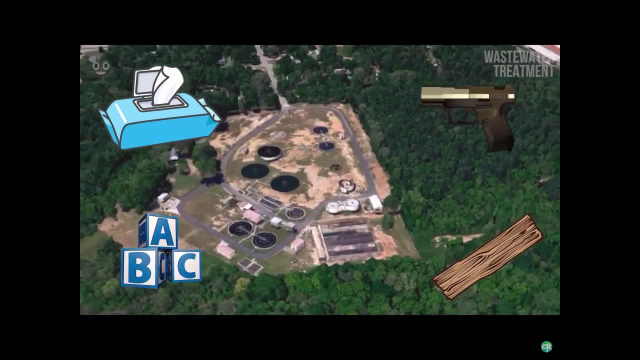 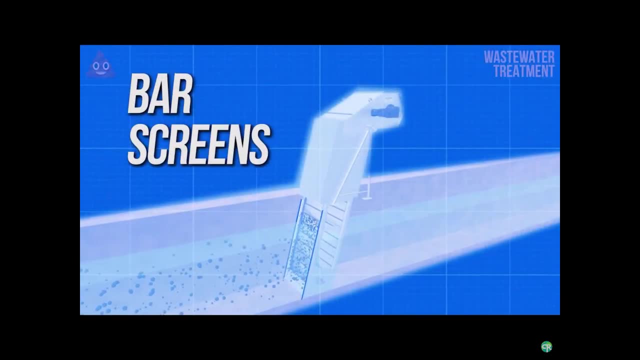 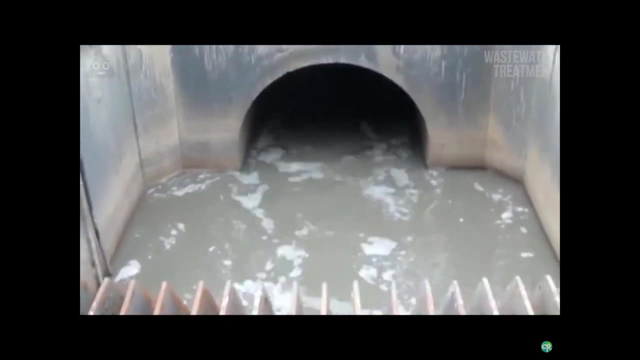 Toe, bar screens, Toys, even guts- You name it- have been caught in a bar screen. Bar screens are exactly what you would think. They are larger vertical bars that stand at the inlet of nearly every wastewater treatment plant. This first process, where bar screens are used for getting to the plant and hurting machinery like pumps. 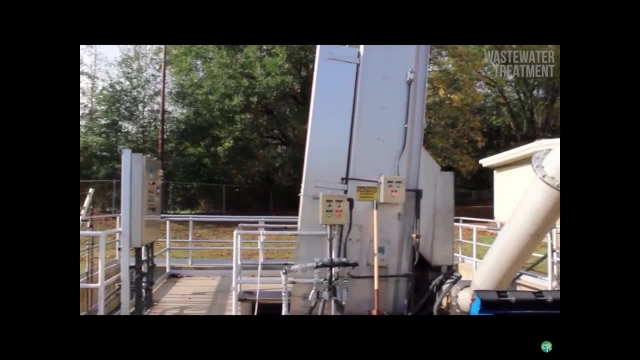 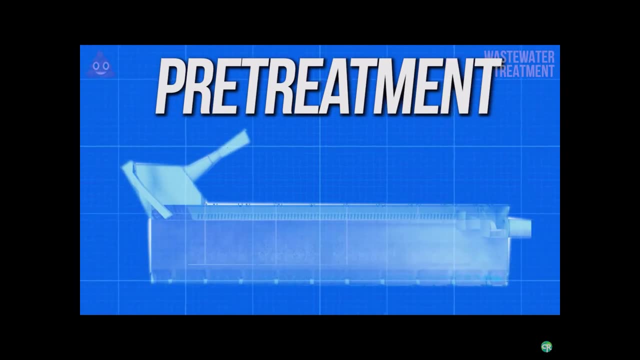 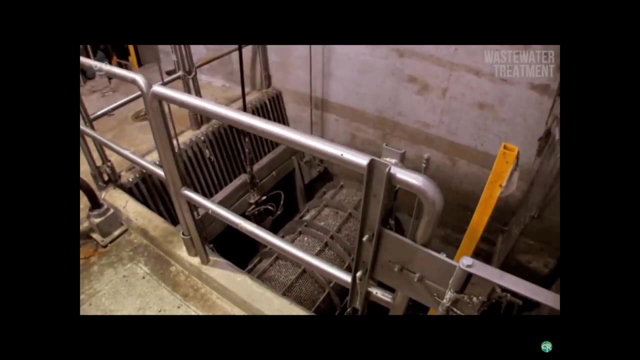 The sole intention of pre-treatment is to remove the outliers in the sewage and make the whole mixture a little more homogenous and in the form of slightly less of chunk treatment. Bar screens are typically mechanically rigged at certain intervals depending upon the flow rates. 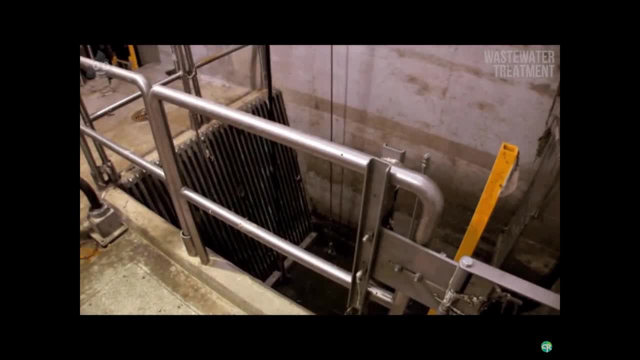 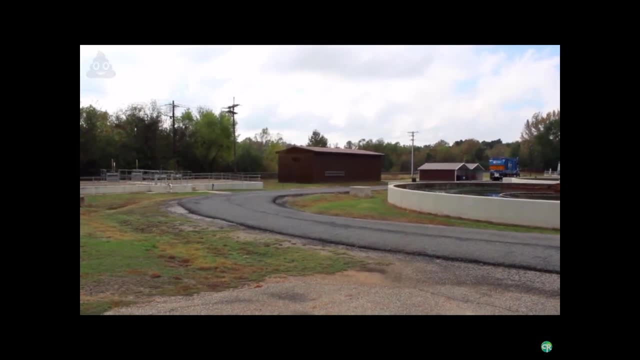 of the water treatment plant- Although some other plants- is then sent off to your average landfill for solid waste handling facility. Whatever is removed from the bar screens is then sent off to your average landfill for solid waste handling facility, Whereas in the case of unusual items. 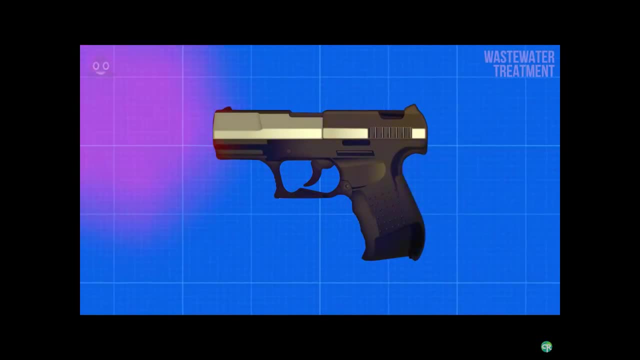 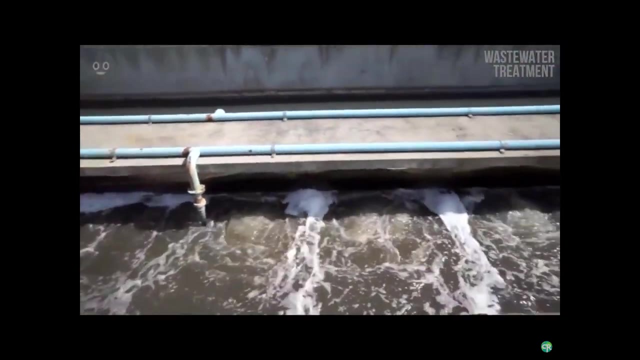 such as guns, they're sent off to the evidence locker in a police station to be investigated. Next up is the grip chamber. Since these bars don't catch everything- larger particles, all grit. Since these bars don't catch everything. as the sewage flows into the grip chamber. 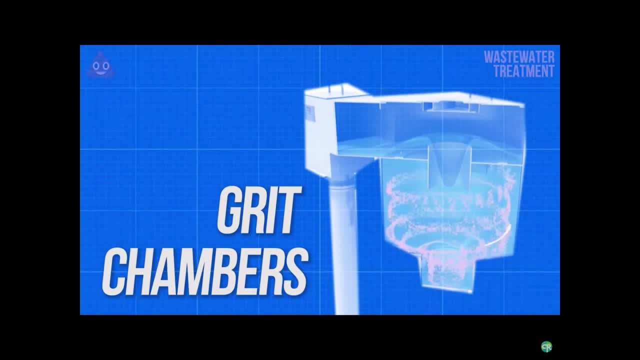 the velocity of the rather viscous sewage is adjusted to allow for particles of sand and rock to settle out. This is needed because these particles can't be removed using chemicals and they could potentially clog or destroy pumps later on in the process. There are three types. 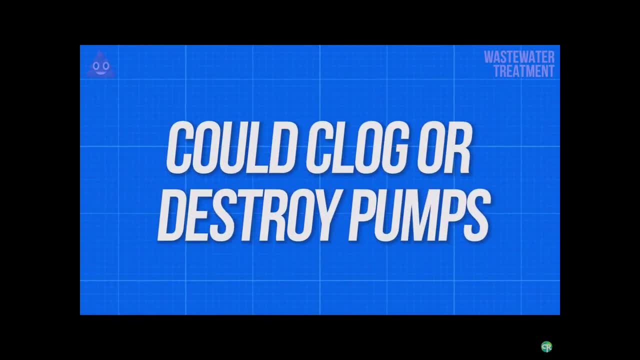 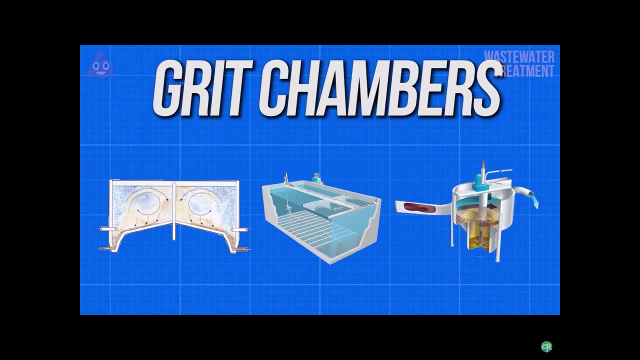 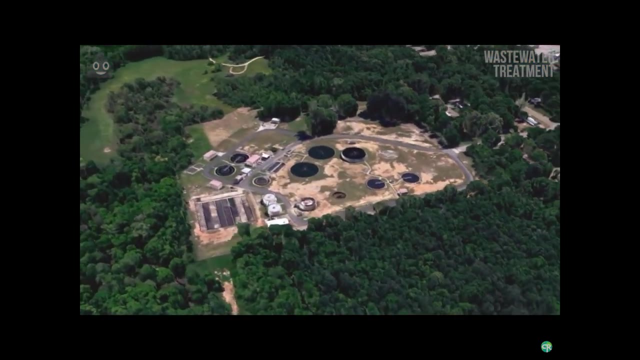 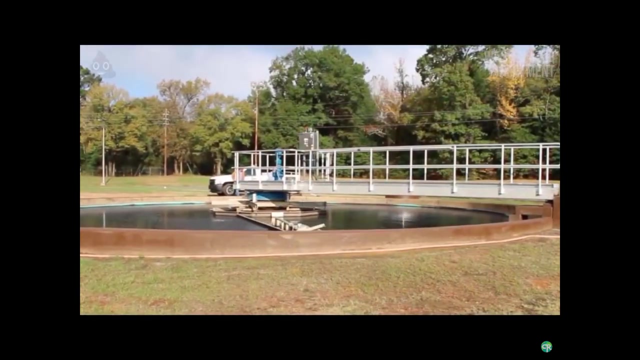 of these chambers: horizontal grip chambers, aerated grip chambers and vortex grip chambers, which all accomplish the same task, as aerated grip chambers and vortex grip chambers, which all accomplish the same task using slightly different methods. bunlar crois, crois. 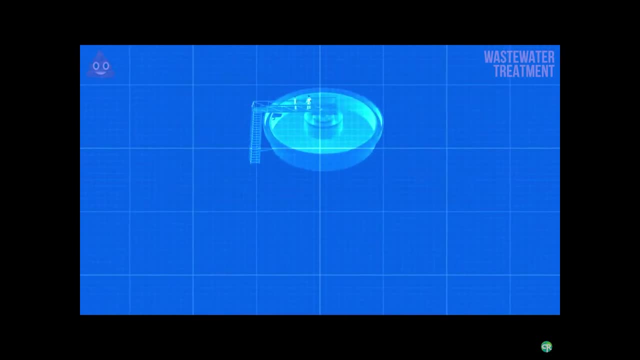 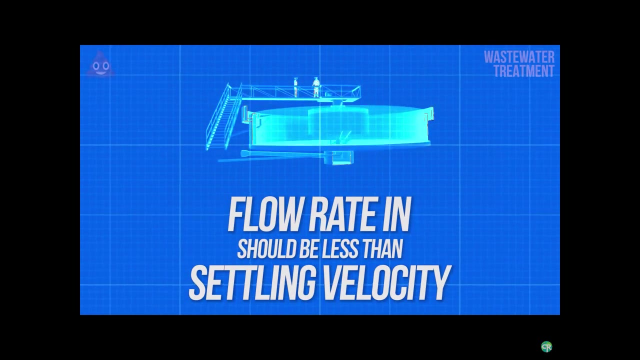 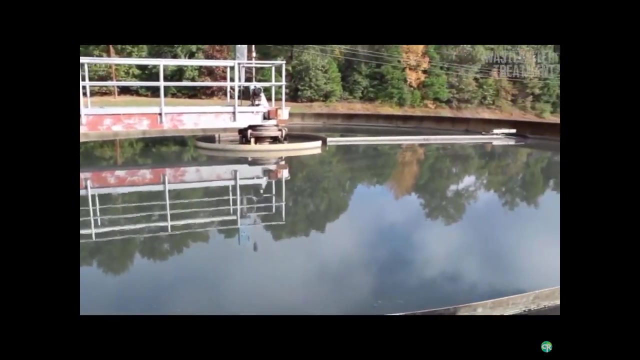 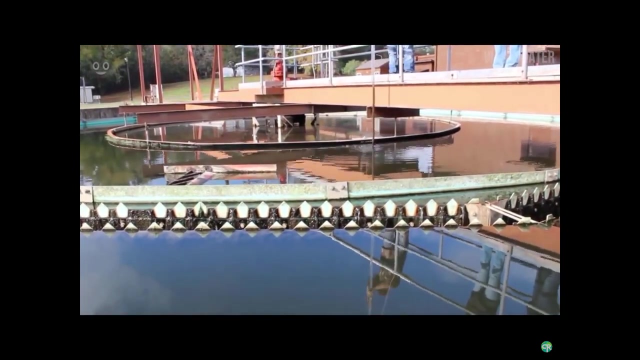 crois policies: causes, causes, causes, causes, causes. In order to accomplish this, engineers will vary the size and number of primary flow flows in accordance with the plans for its flow rate. This ensures that, at this step in the process, solids can settle out of primary clarifiers with the correct quantities. 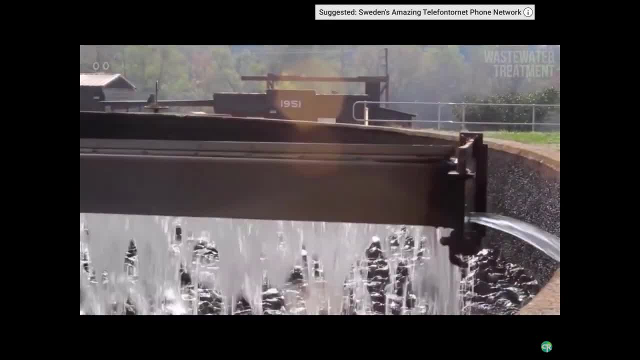 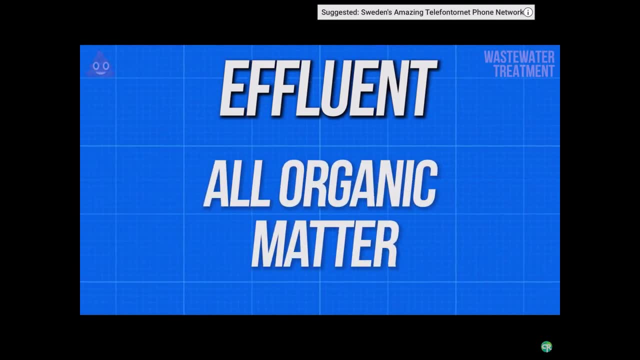 At this step in the process, microliters and should be all organic matter which will be treated further. The top layer of the microliters and should be all organic matter which will be treated further. The top layer of the clarified water flows over a clear wall into the next basement. 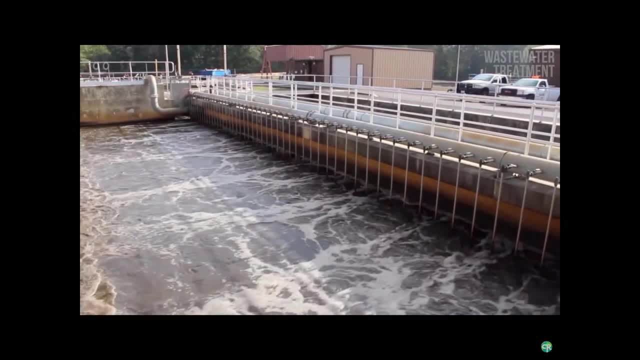 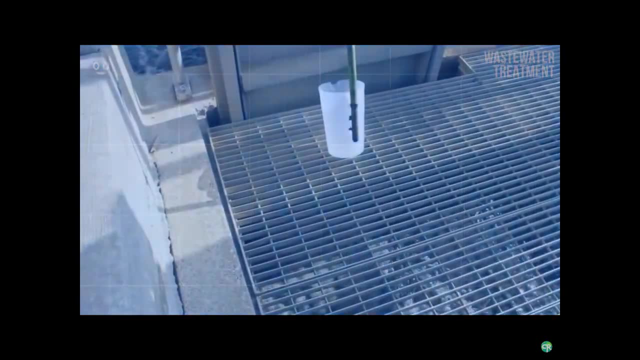 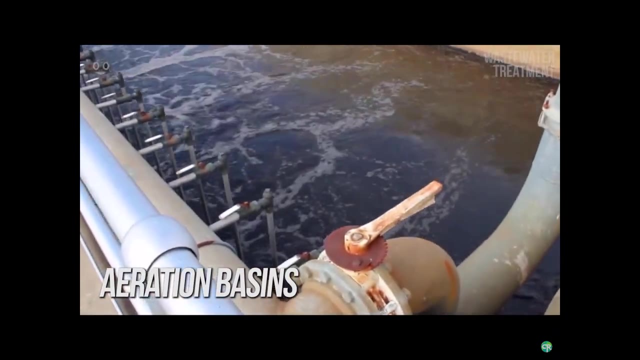 The sole focus of which is to significantly degrade the biological content of sewage. In many cases, this process starts with aeration basis. In many cases, this process starts with aeration basis. Eflin flows into the aeration basis, at the bottom of which are hundreds, if not thousands, of tiny air blowers that create bubbles in the water. 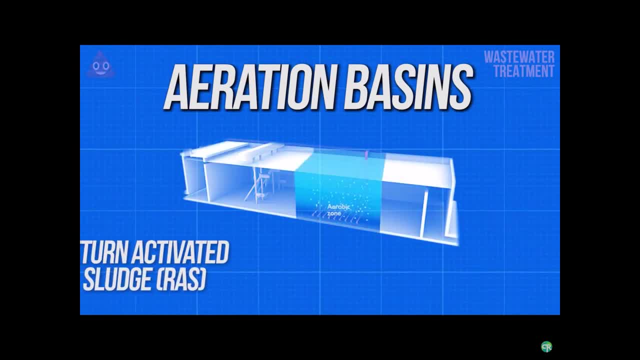 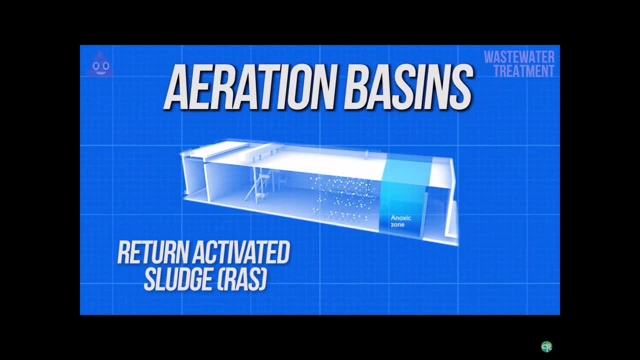 You could think that this kind of activated sludge is a bunch of sludge. This introduction of something called return activated sludge. You could think of return activated sludge as a bunch of significant amounts of bacteria, along with the massive amounts of oxygen injected from the bubblers. 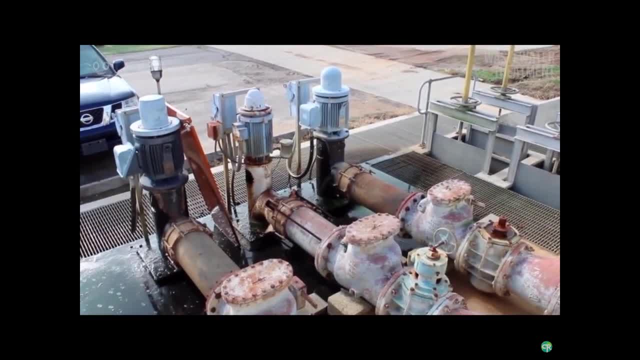 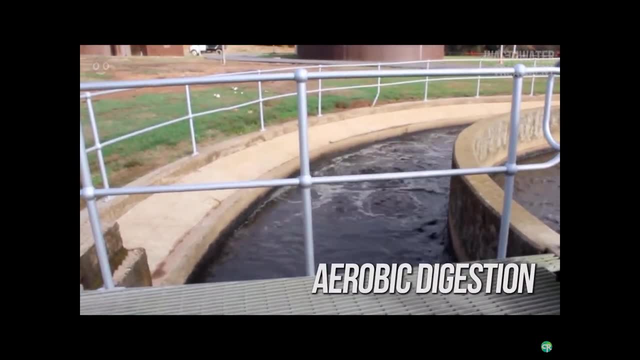 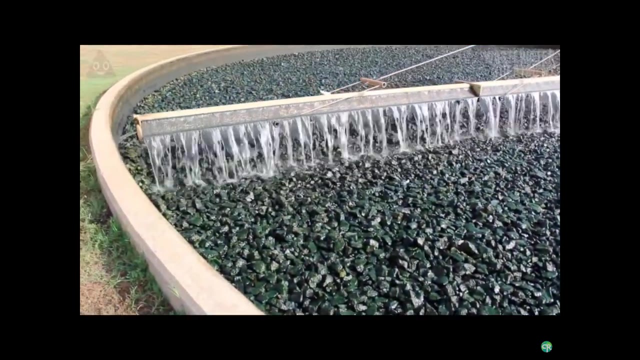 This introduction of significant amounts of bacteria, along with a massive amount of oxygen Injured from the bubblers, creates the amount of organic matter along with the use of excess oxygen. Some older plants will add in another step of aeration basis, referred to as bio crochets or Trem globalization. 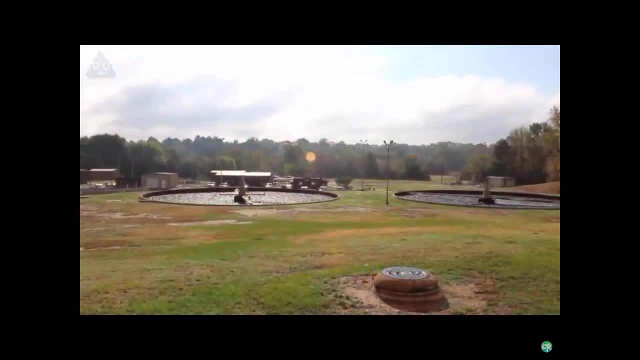 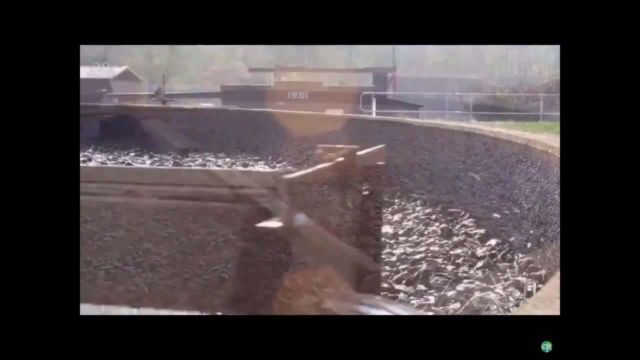 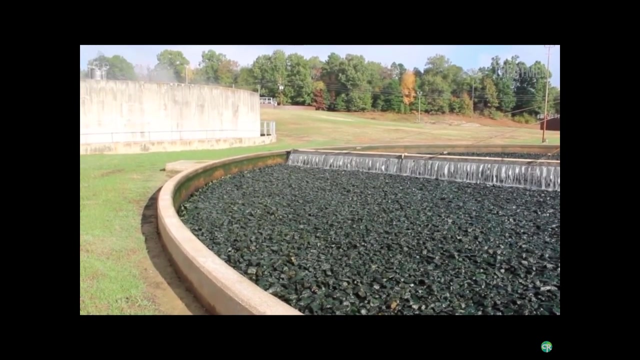 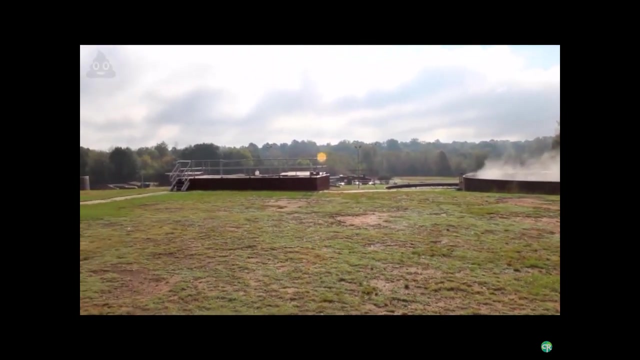 This step is largely not for a film of bacteria to chow down on any organic matter in water. This step is largely not used in newer plants due to more efficient and effective water processes, but for plants with bases already installed. Many still use them because they only benefit the treatment process into a secondary filter. 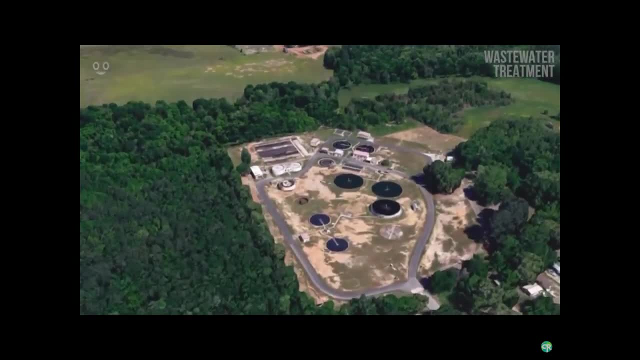 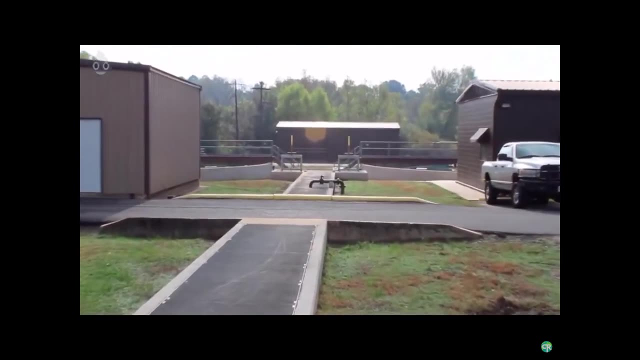 or clarifier, where some of the sludge, along with much of the sludge, is pumped into the aeration basins as the return act of the sludge, Further settling of larger particles is also accomplished in these basins, as it is the final step of the process that will remove solids and larger biological matter. 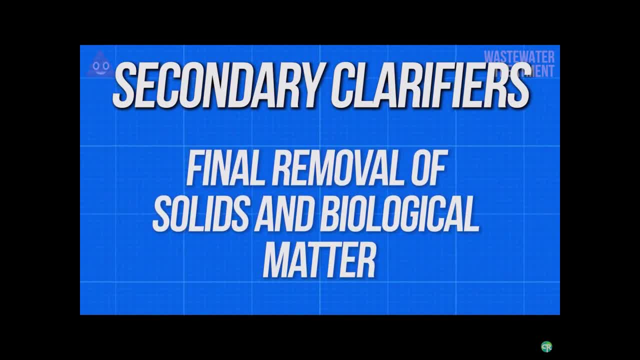 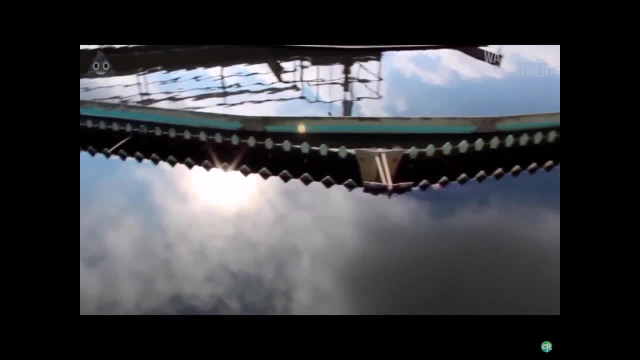 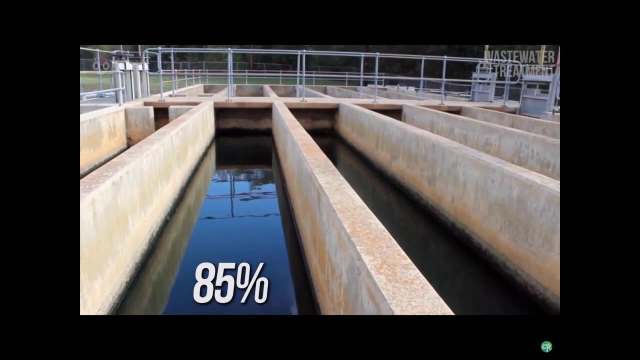 Water flows out of secondary clarifiers over a nearly identical weir wall to the primary clarifier and moves on to the disinfection process. At this point, 85% of all organic matter is removed from the water process. At this point, 85% of all organic matter is removed from the water and the effluent. 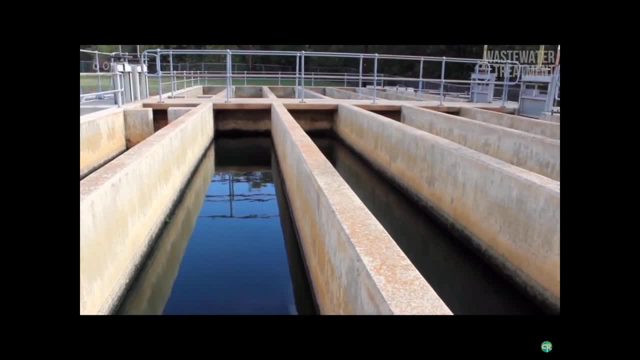 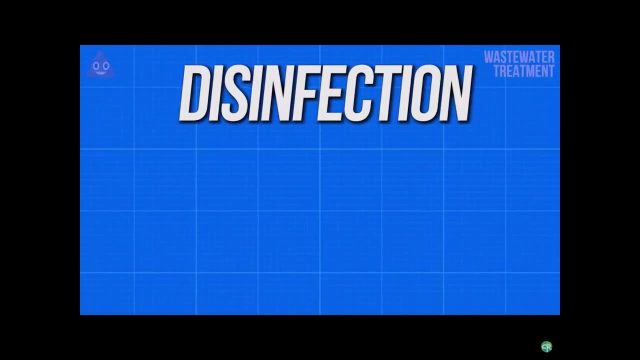 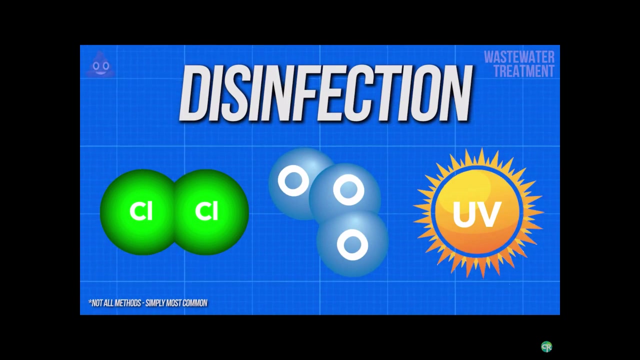 should be safe to drink in most cases, although you probably wouldn't want to. Disinfection is the final step of the process and is usually accomplished in one of three ways, either through chlorine, ozone or ultravital disinfection. Each process has its benefits and drawbacks, with each being used commonly throughout the 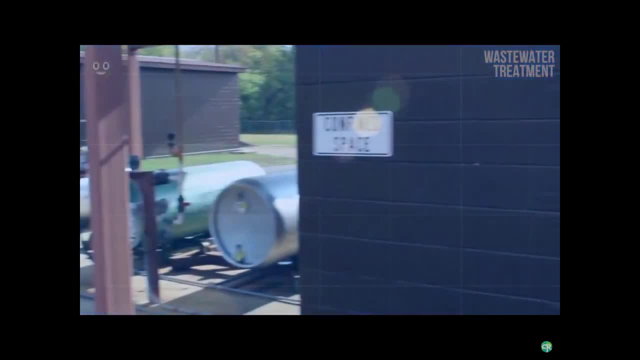 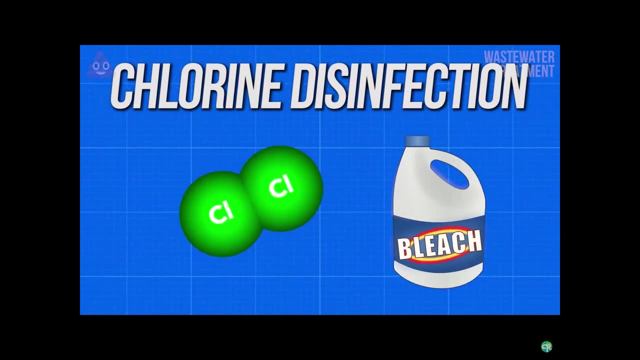 wastewater treatment process across the world. Chlorine disinfects the water. chemical disinfection Chlorine, which you can think of as concentrated bleach, is added to the effluent here to kill off any remaining bacteria and organisms still living in the water. When 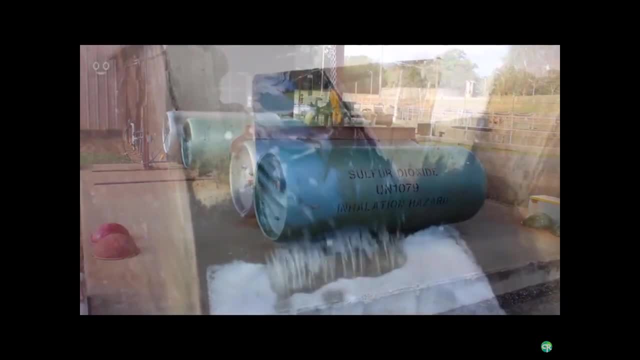 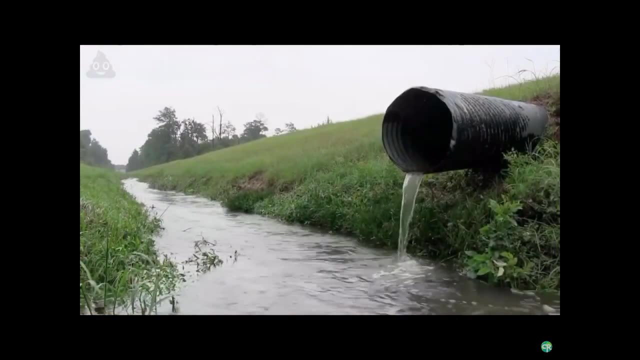 chlorine is added to kill off the bacteria. it then has to be removed, or it can be discharged just to not kill off anything in the discharge location. After this, the water is safe enough to discharge into an electrical current. Ozone disinfection is another method of disinfection. 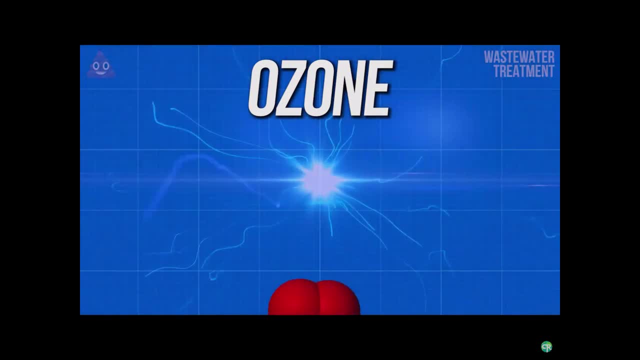 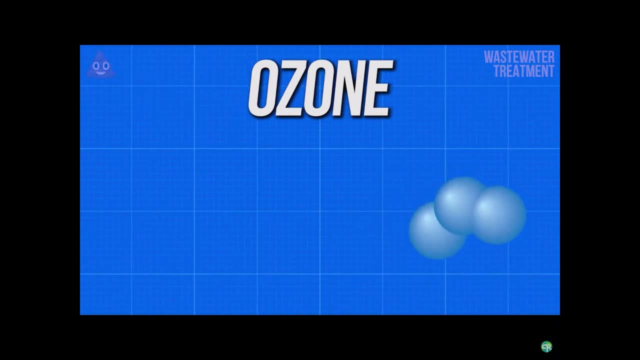 that involves pumping an electrical current through the water that causes oxygen molecules to disassociate and combine with a free oxygen molecule, forming O3, known as ozone. Ozone is an incredibly strong oxidant that causes microbe cell walls to leak- Rapid cell decomposition. 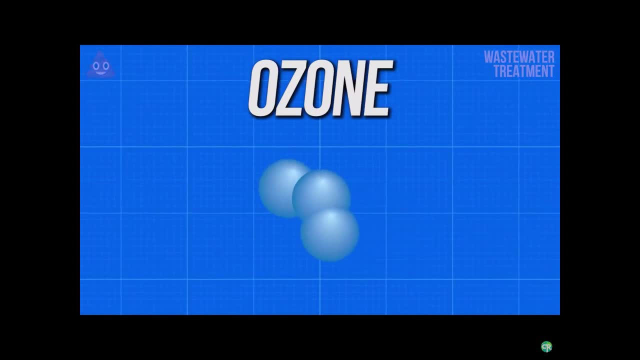 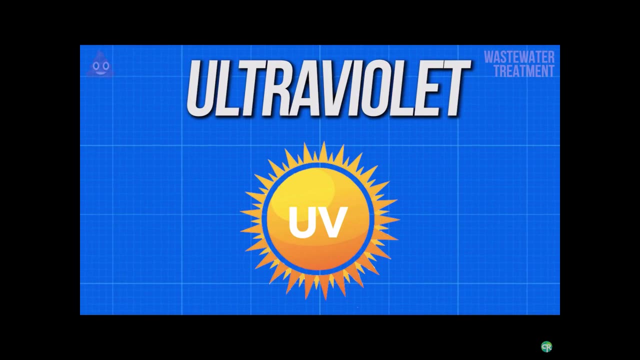 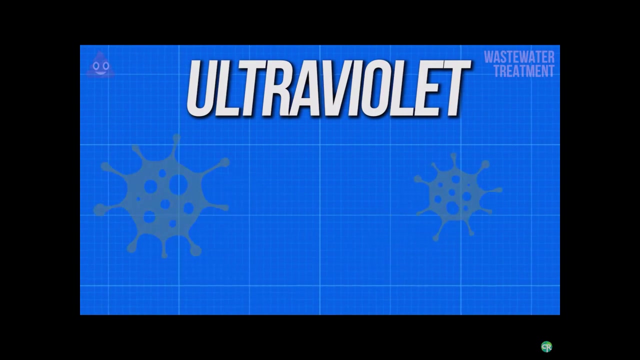 can cause overall damage to cells. In other words, it kills off bacteria. The last common method uses ultraviolet light to scramble bacteria's DNA so that they cannot multiply. In UV disinfection, bacteria or water aren't killed, rather, they're sterilized, rendering them harmless. If you were to 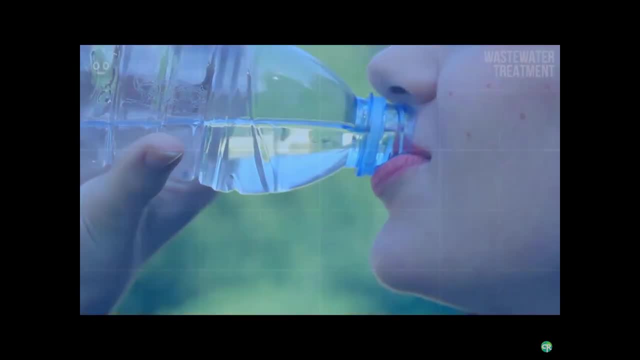 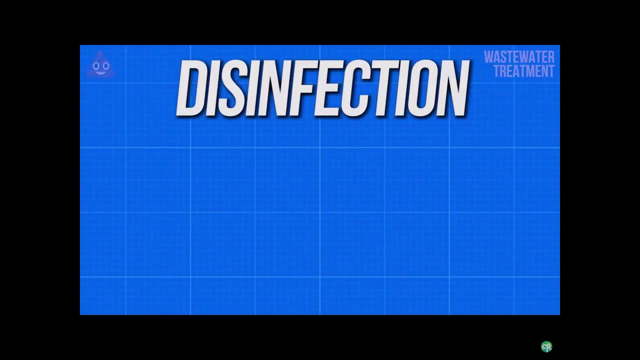 ingest water with living microbes immediately following UV treatment. any harmful bacteria would be unable to multiply or render your body damaged. Engineers choose between these methods based on a variety of factors such as flow rates, cost and location of discharge, which brings us. 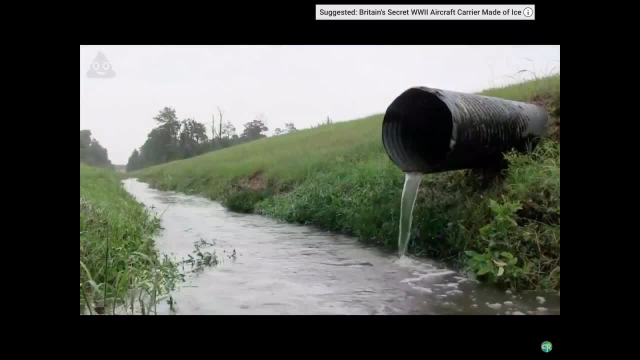 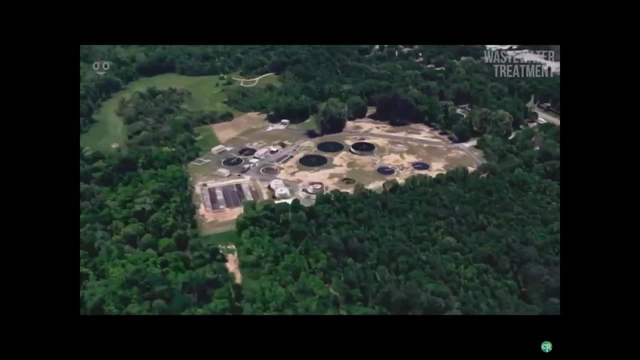 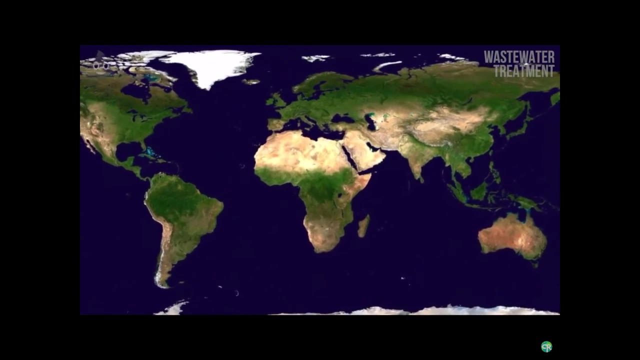 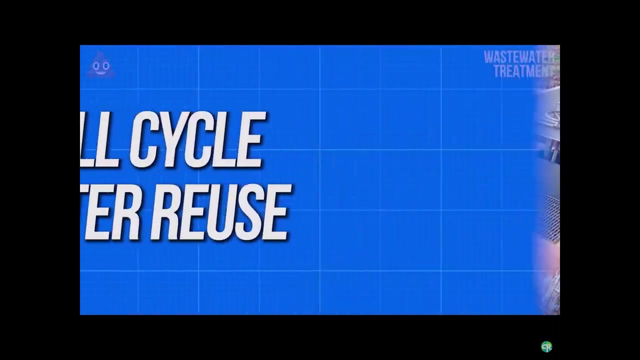 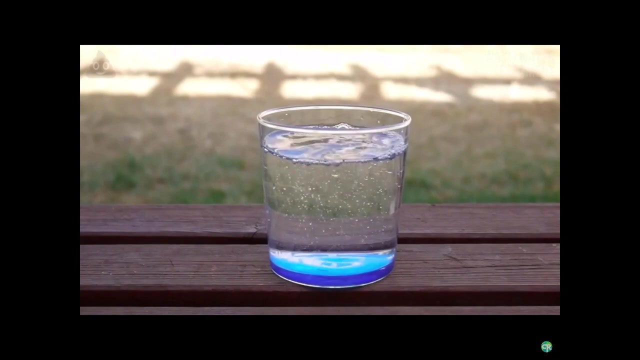 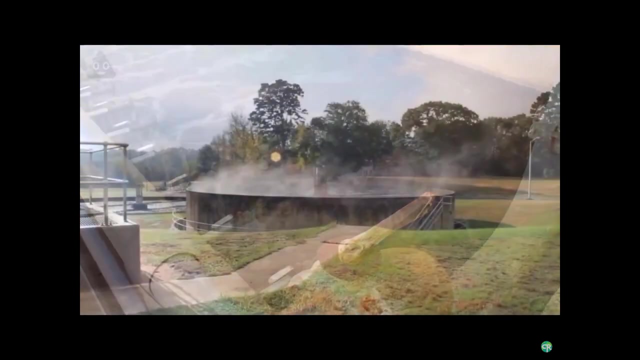 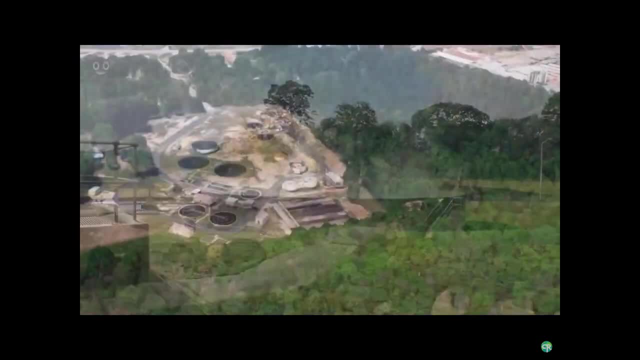 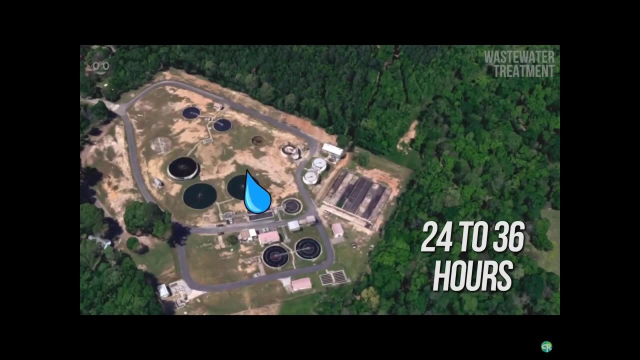 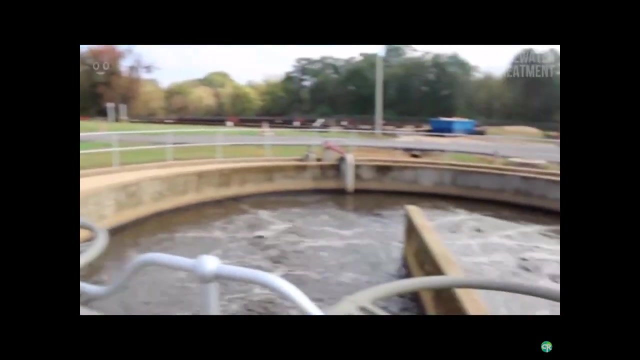 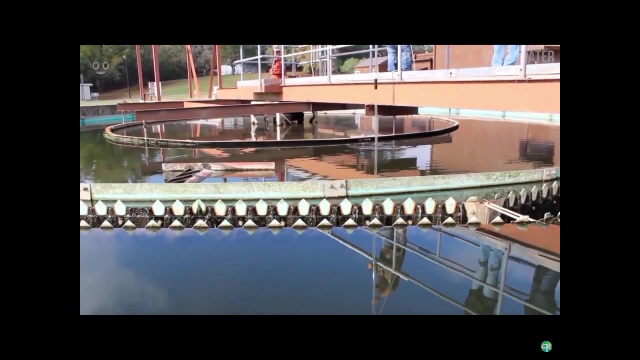 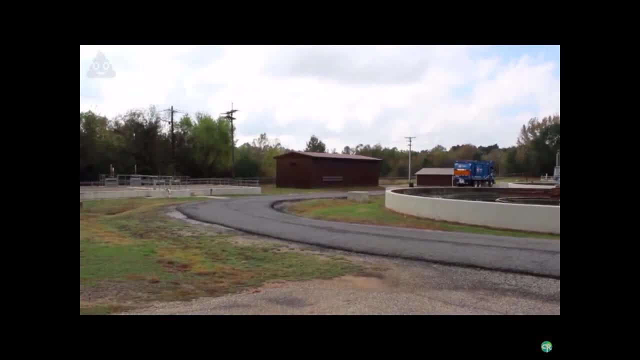 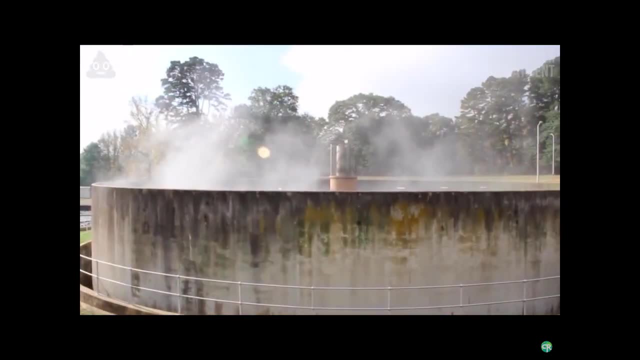 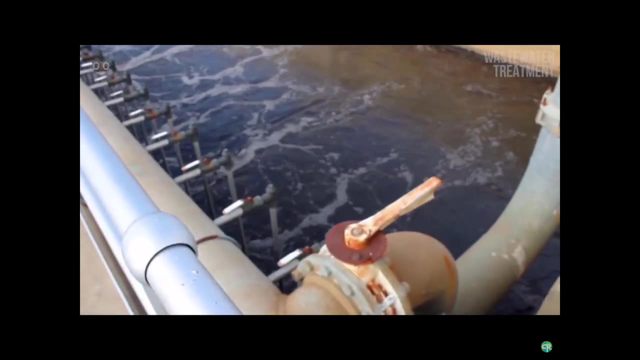 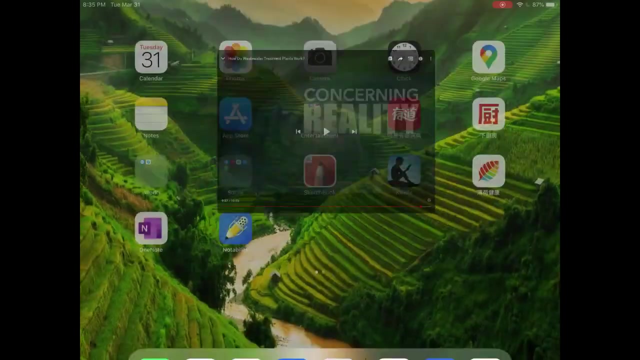 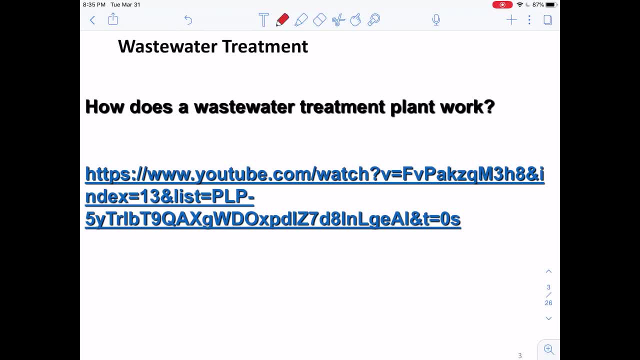 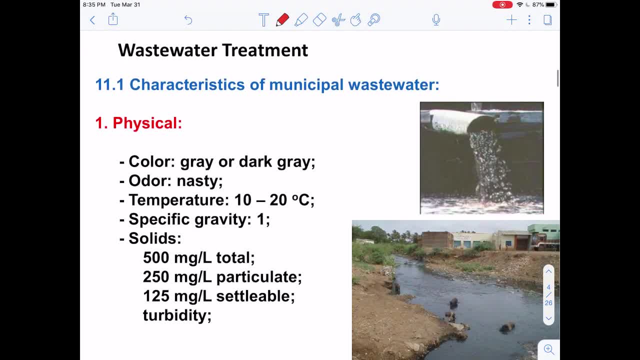 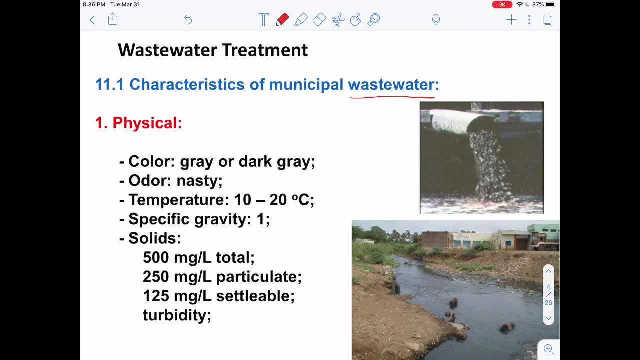 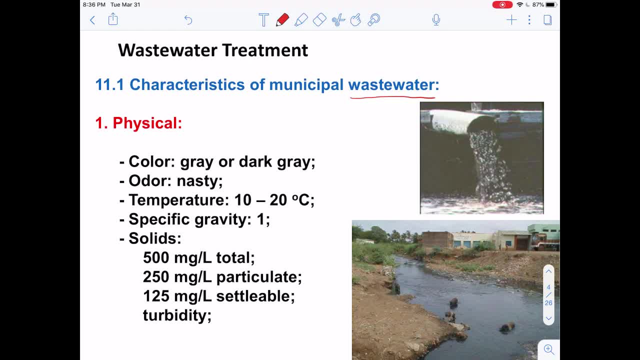 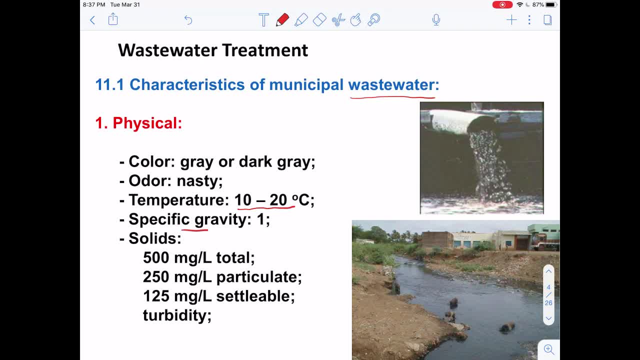 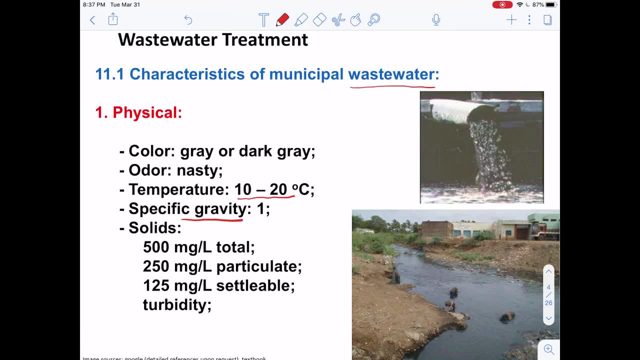 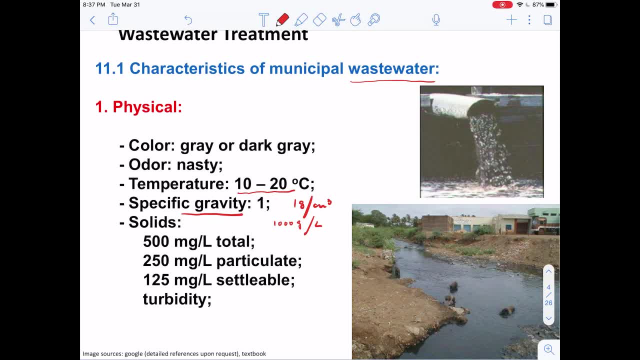 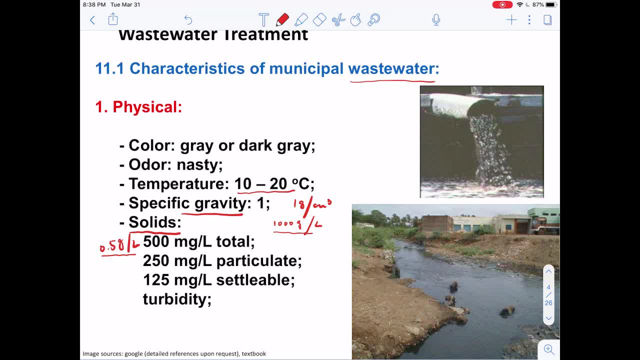 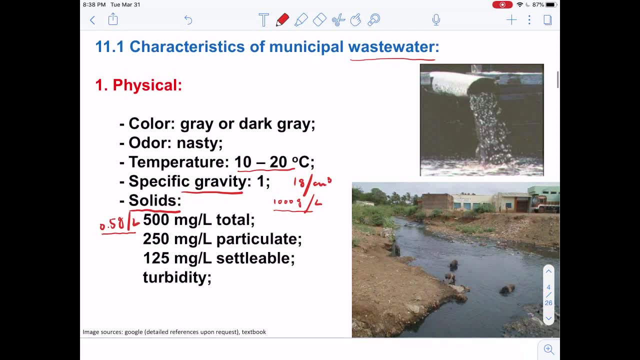 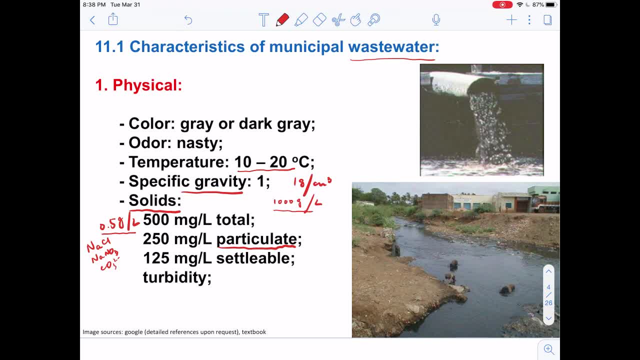 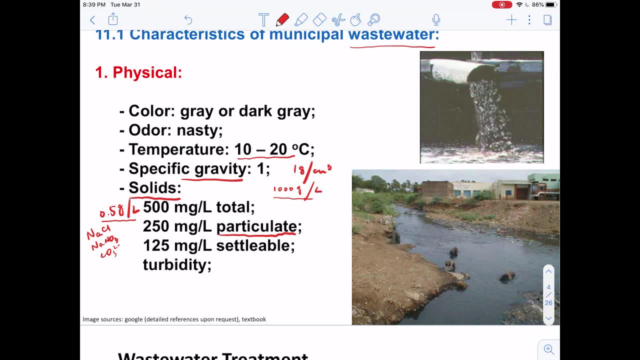 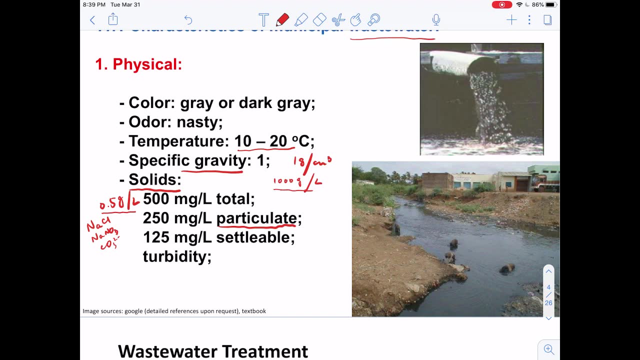 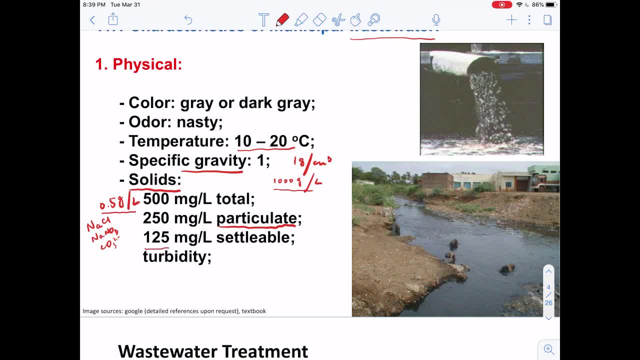 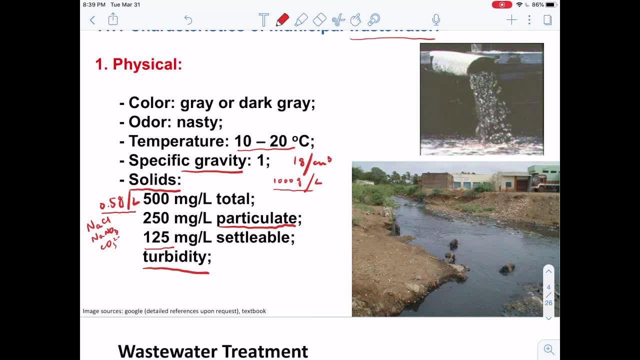 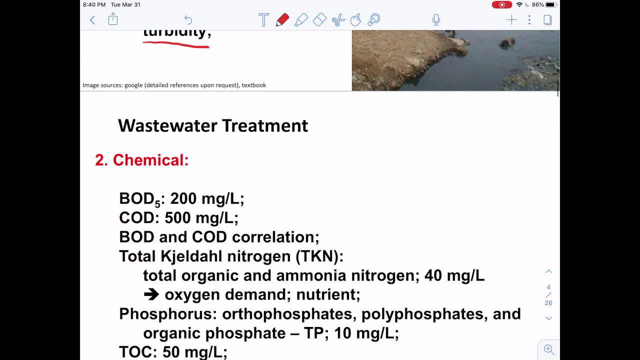 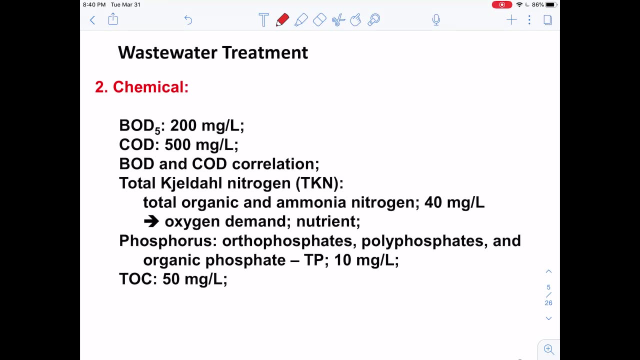 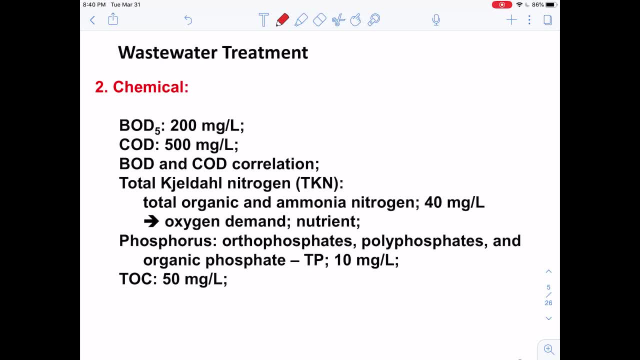 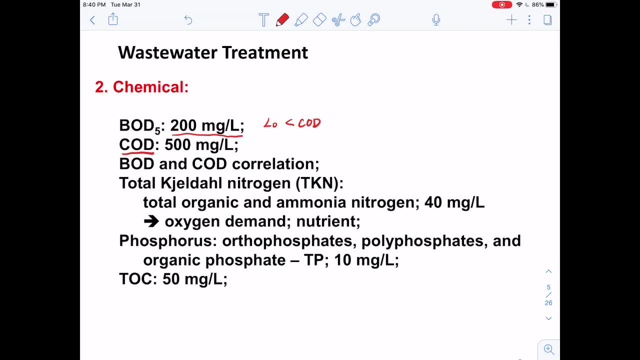 than COD, which is mainly because part of these organics are being used by the microorganisms to construct themselves right and they're not in. the microorganisms are not going to consume all of those organics because they're also emitting organics or that they cannot process into the water. so that is. 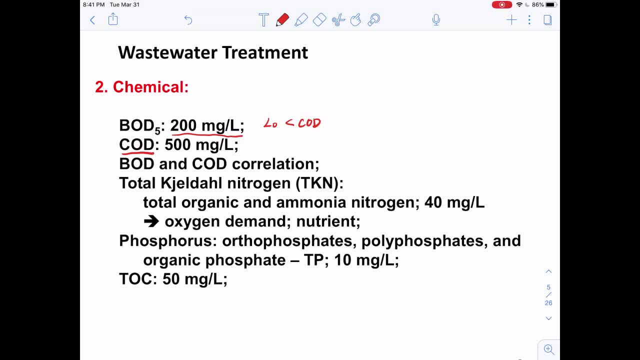 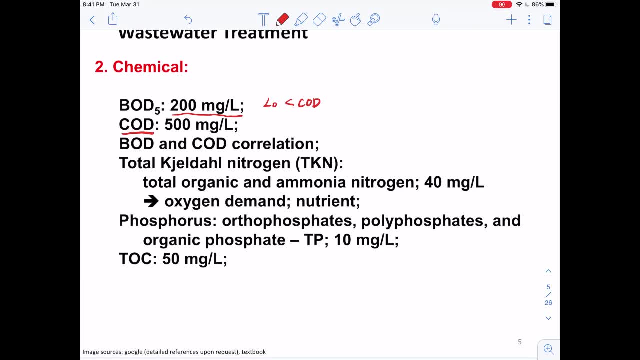 why the ultimate BOD is going to be smaller than the COD there and therefore there is a correlation between the BOD and COD. and in terms of the nitrogen contents, typically we will use the total culdo nitrogen, or the TKN, to describe the nitrogen concentration in the water, in the wastewater. so these nitrogens- 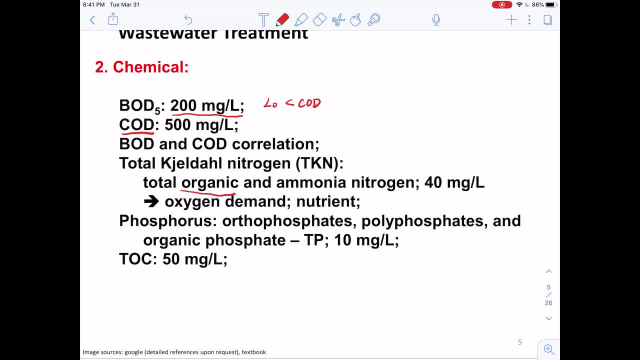 will exist in the organic contents, organic form, and also the ammonium form, ammonia form and typically for the municipal wastewater they have a TKN of around 40 BOD milligram per liter. so we want to treat these nitrogen. on one hand, it's because these nitrogen will actually demand oxygen right we talked about in the NBOD. 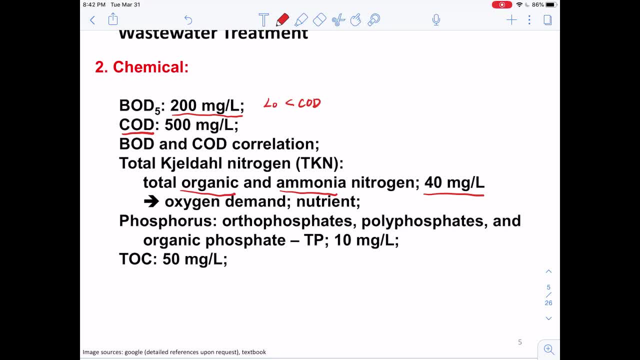 in our last chapter. so these will remove, or these will reduce, the dissolved oxygen in the water but on at the same time, the nitrogen will exist as a nutrient right so they can be utilized by the algae which is causing the algae bloom, and that will further reduce the water. 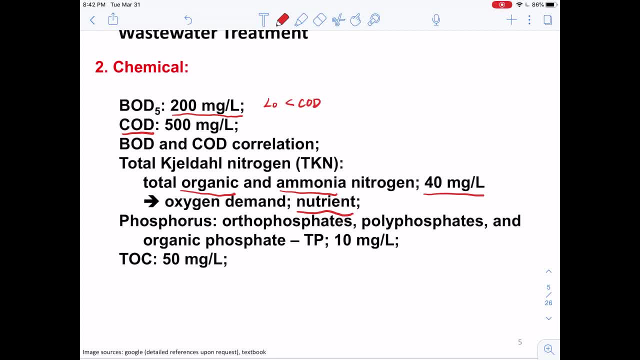 by forming a lot of biomass there. in terms of the phosphorus, the phosphorus can exist in the autophosphates, polyphosphates and organic phosphates. now we call these phosphates as the total phosphorus, or the TP, and for the municipal wastewater they have an average concentration of around 10. 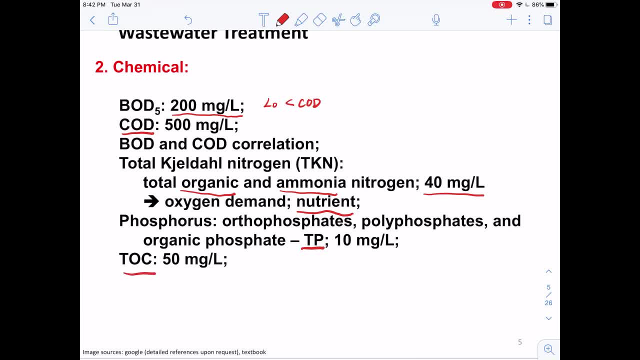 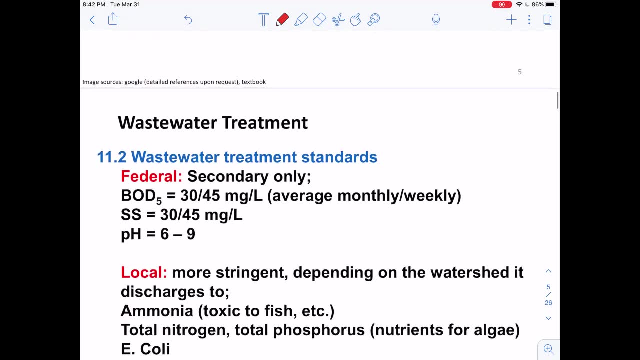 milligram per liter. so this TOC here means the total organic carbon, and they normally have a concentration of around 50 milligrams per liter. so we want to treat as much as possible, which is around 50 milligrams per liter. okay, so these are the characteristics on the chemical side of the municipal wastewater and the 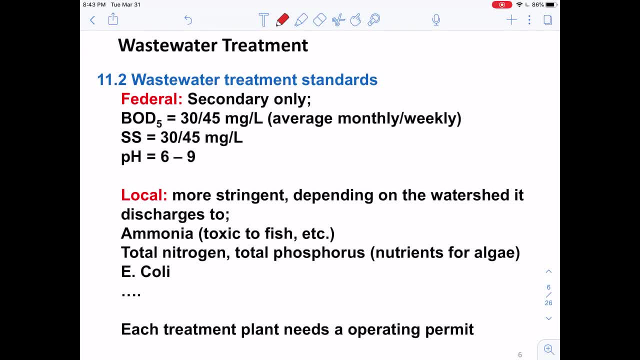 reason why we want to treat the wastewater quality is that people set up standards right. we don't want to emit all of these wastewater into the environment and that is causing hazardous or the hazards to the ecosystem. so that's why we set up these standards and the reason we want to treat. 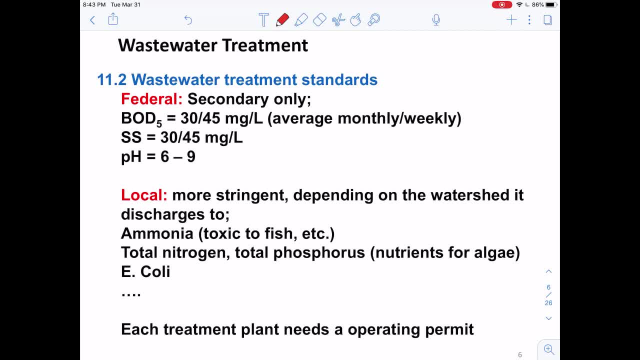 and so, then, we need to know what are these standards? briefly, and there are standards for both the federal level and also for the local level. in terms of the federal level, they will require that the wastewater treatment will need to go through secondary treatment. okay, so later we'll find out that for the water treatment and wastewater treatment, we have the pre-treatment. 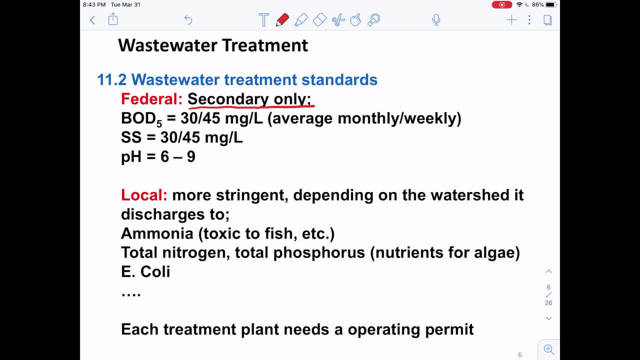 process, primary treatment process and also the secondary treatment process and for the federal requirements we need to do all of these okay, so there can be tertiary, tertiary treatment, which is further higher levels of the treatment. but in terms of federal level we need to do until secondary uh treatment process okay, so the federal level regulates that for the bod5. 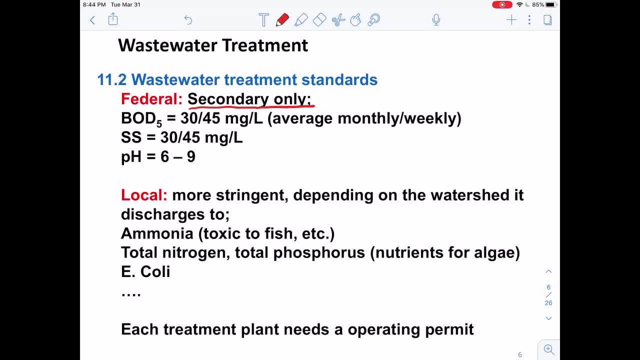 you need to satisfy the monthly or weekly limits here. okay, so the for the monthly limits is around 30 mg per liter, while for the weekly limit it is 45 mg per liter. so what that means is that if we measure the bod5 every day and if we average the bod5 concentrations over a whole week, then the 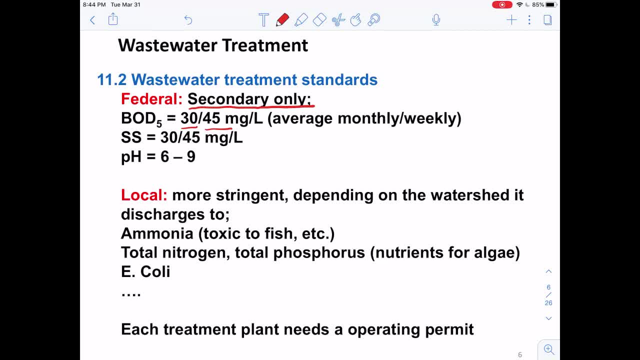 concentration or the bod value. bod5 value have to be lower than 45 over a whole week and has to be lower than 30 over the whole month. so you may wonder why are we having different standards for the weekly or monthly requirements here? so this is actually considering the fluctuations in the emission of 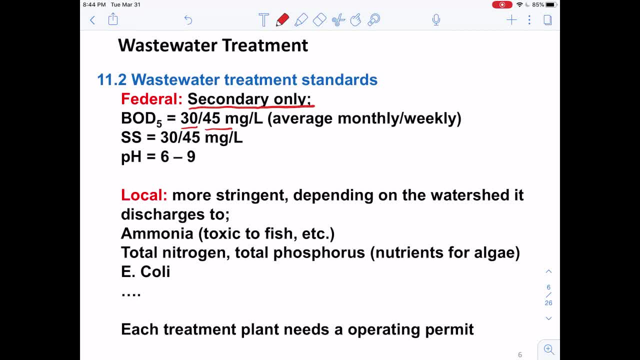 these bod or these oxygen demanding materials, for example, if we plot out the emitted bod as a function of time, so there can be a really low concentration and there can be also high concentrations here, right? and this higher- lower concentration is not stable or is a very random, because it really depends on how people consume the water, right? so let's say that. 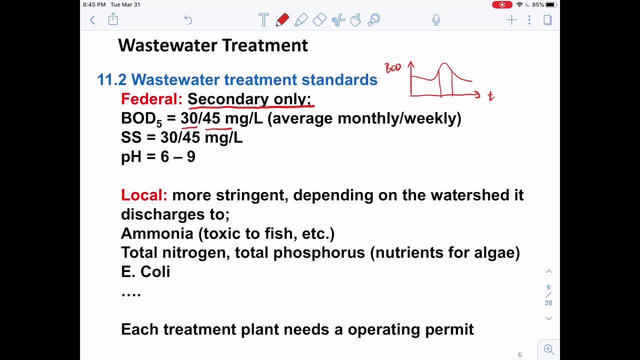 if we measure the bod concentration over this entire week here, let's say that this is seven days. so as long as this average concentration which is around here is below 45, then we'll say that, or below 45 milligram milligram per liter, then we'll say that the water quality is good. enough because there are also low concentrations. for some years, 1, 0 below 45- things are good enough because there are also very low concentrations. so that is why that is so that we have to check these jektional: what an average, goddam, concentration level. and then we'll say: that is really, that there is very good. 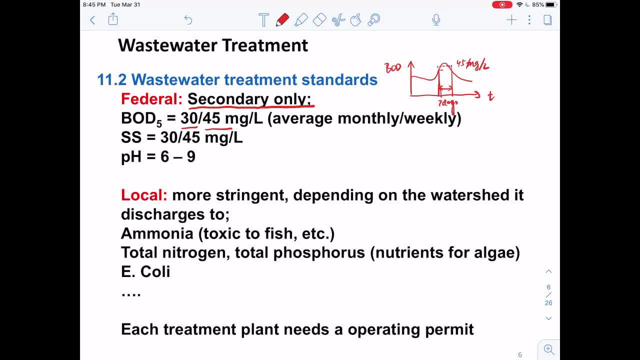 concentrations over the rest of the month here, right? so if we look at the average concentration over the whole month, then it might look like this: okay, so this will also satisfy 30 milligram per liter. so that's why we set up different standards for different averaging times here, so this also. 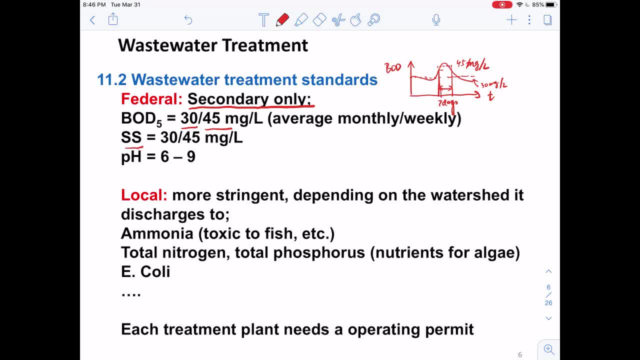 happens for these suspended solids, like the SAS here. so for the suspended solids. and then the average monthly concentration needs to be lower than 30 and the average weekly concentration need to be lower than 45, and in terms of the pH, the federal limits regulates that pH have to be within the range between 6. 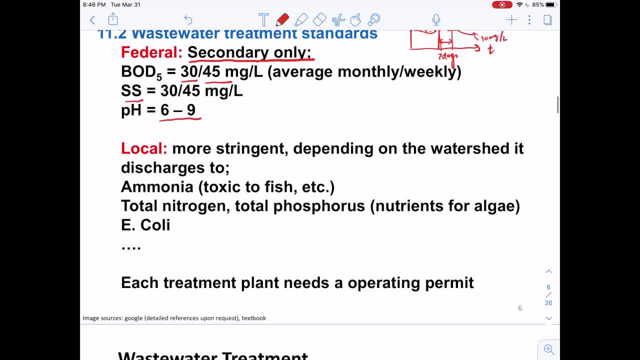 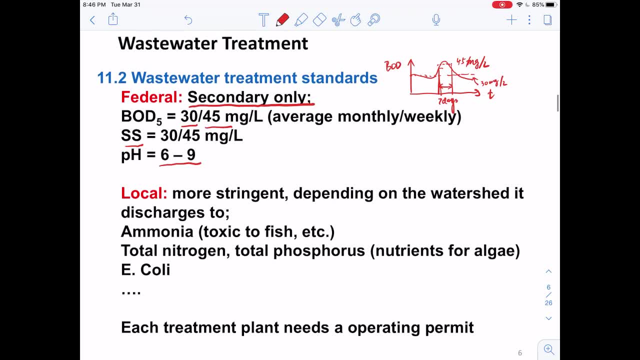 to 9 and further in terms of the local level. people will put more stringent requirements in terms of the wastewater quality, because it really depends on what type of watershed is going to discharge to, because if the ecosystem in that watershed is very fragile, then we have to put on some more stringent requirements to avoid or to prevent the 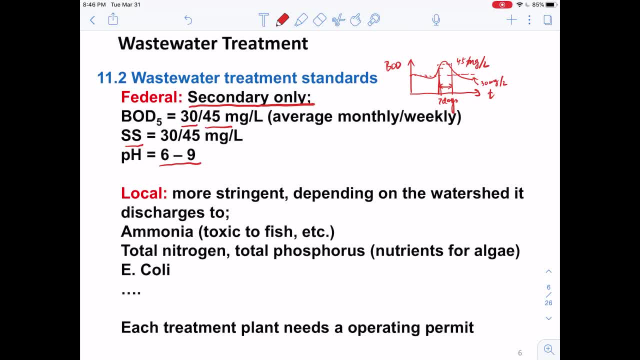 the damage to that ecosystem. so for these local levels we may put into more limits in terms of the water quality. for example, we will require the ammonia concentration, the total nitrogen concentration, phosphorus concentration and even the Ecoli concentration. okay, for these treatment plants, that's treating the water quality or the 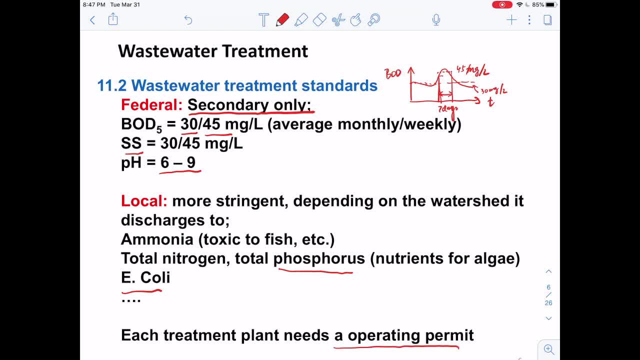 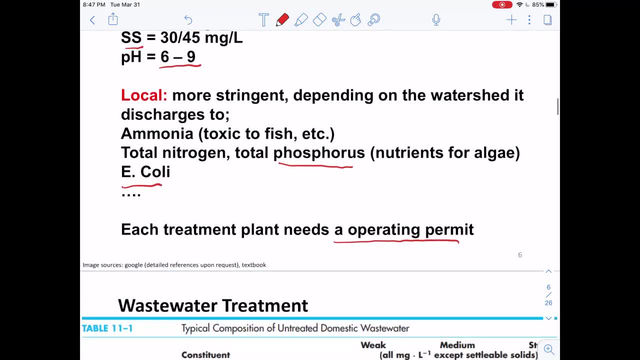 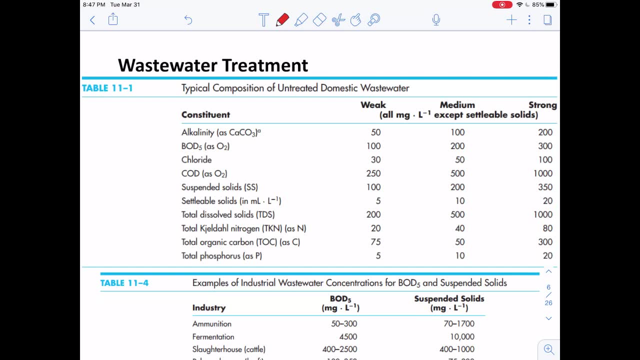 wastewater quality. they will need an operating permit, okay, and also they will obtain those standards from the EPA, as has been shown in the video there, okay, so here I'm listing a few tables regarding the what is the typical concentrations of these contaminants in the municipal water and also the 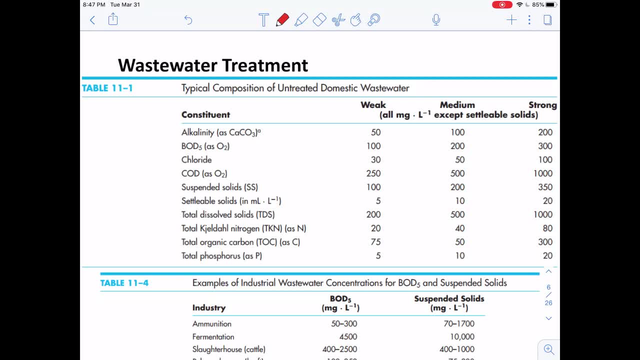 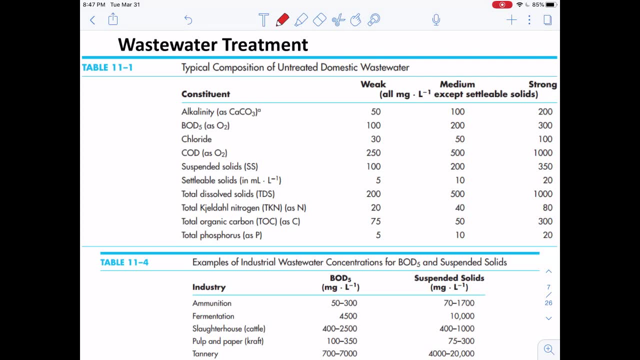 industrial emitted water and also what are the EPA regulations. so here is showing. the first table shows the typical composition of the untreated domestic wastewater or the municipal wastewater. so actually people will use different standards or different categories to describe the wastewater quality, so we can have the weakly. 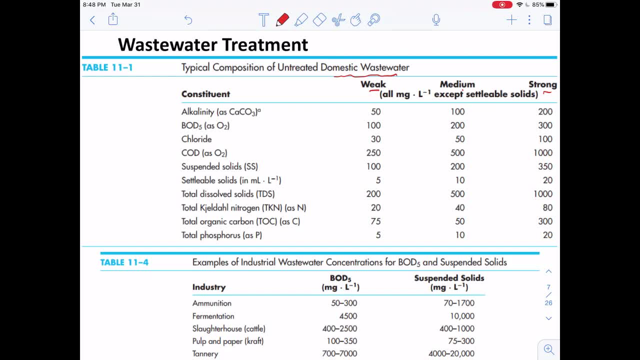 polluted wastewater, medium-level wastewater or strong or strongly polluted wastewater. for different categories, they will have different concentrations of these constituents, For example, for the BOD5 or the suspended solids. you can see that mentioned that it's around 200 for the BOD5 or 200 for the suspended solids. Those are among the 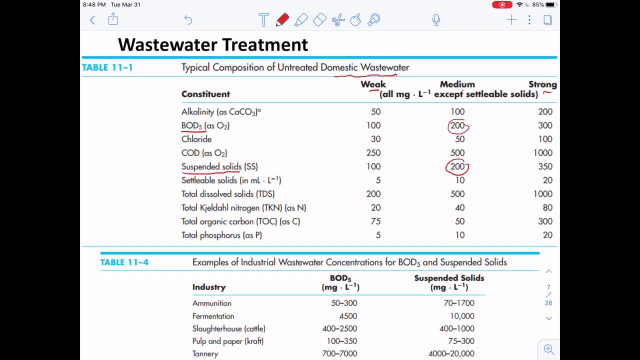 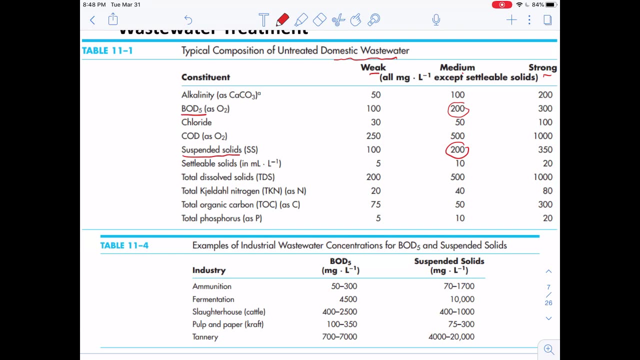 medium levels here. For the weak, weakly polluted water, they may have a lower concentration of these constituents, right, And this is the municipal wastewater. In terms of the industrial wastewater they may have, they will have very different concentrations of these pollutants because really depends on. 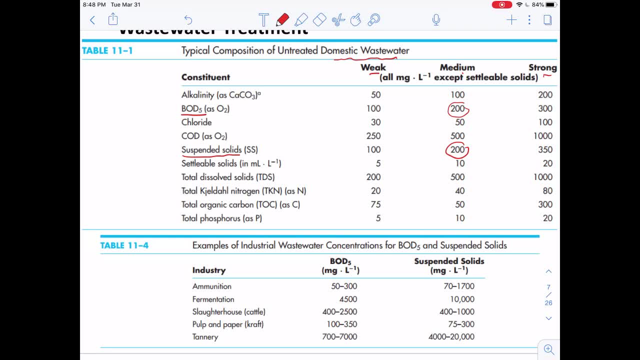 which type of industry we're talking about, Because different industries, they will process their chemicals or the resources differently and their wastewater properties will also be quite different. For example, if we're talking about the fermentation industry, then they will typically have a very high 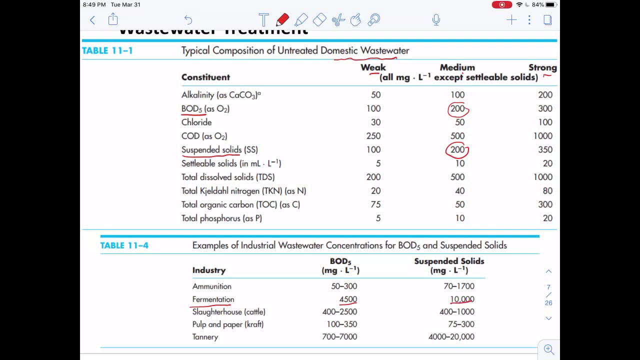 BOD5, right, And also the suspended solid concentration will be very high too. If we're talking about the slaughterhouse there, then the BOD5 really depends on what is the typical operating periods? right? Because they're not. they're not operating the plant under a steady state condition And we need to. 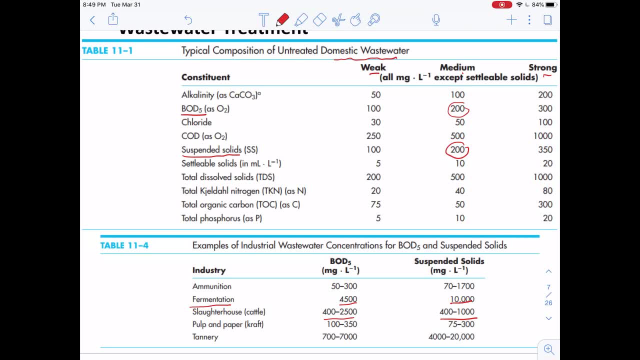 talk about the demand and supply, so there's always a range in terms of these water quality here And, as you can see, for the industrial wastewater they will have much higher concentrations of these pollutants or the constituents. So that's why we need to put in more stringent requirements for these. 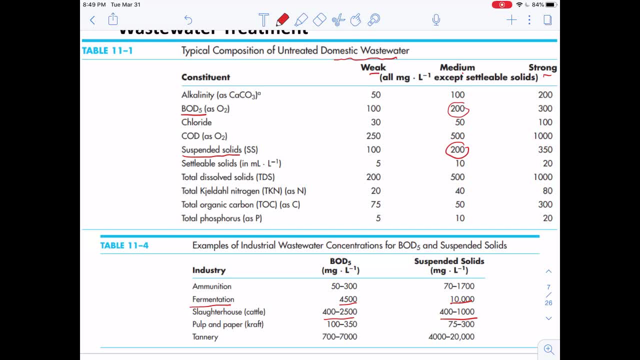 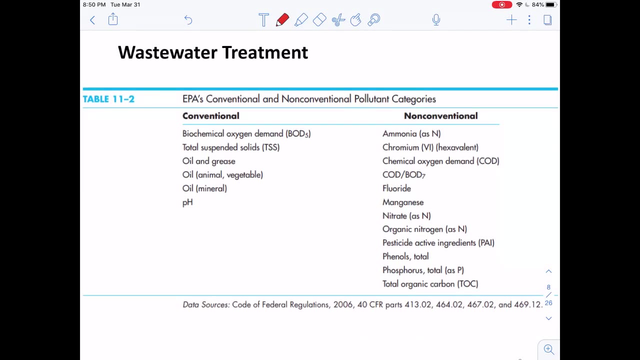 industrial plants so that they can purify their water before they emit them, before they dump them into the nature here. okay, So here is a table that's showing the EPA requirements in terms of the different constituents of the water. So there are conventional requirements, right? or the conventional pollutant. 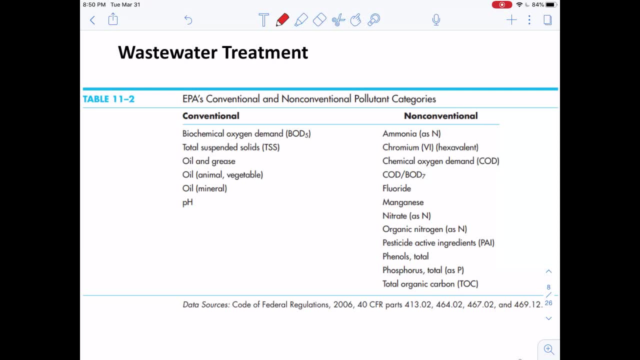 categories, which includes the BOD5, total suspended solids and also the oils. You can see that there are different types of the oil too, and also the pH, which we are quite interested in, And in addition, there are non-conventional. 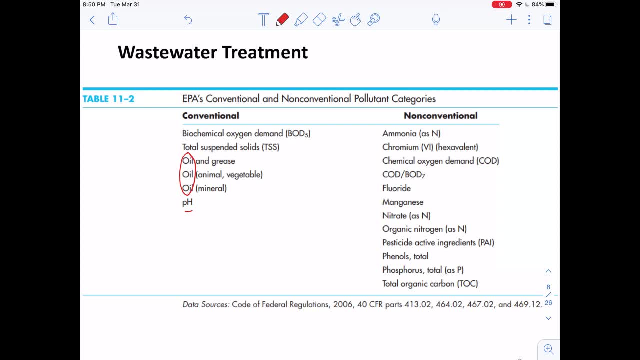 pollutant categories, which is a broader spectrum of these requirements, which will include, let's say, the COD, BOD7, right? So other types of chemicals, ammonia, fluoride and manganese, so on and so forth. okay, 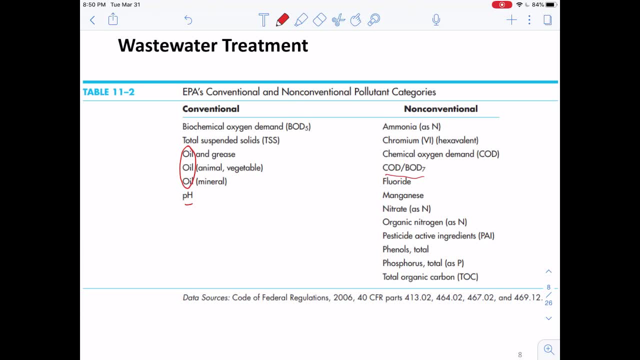 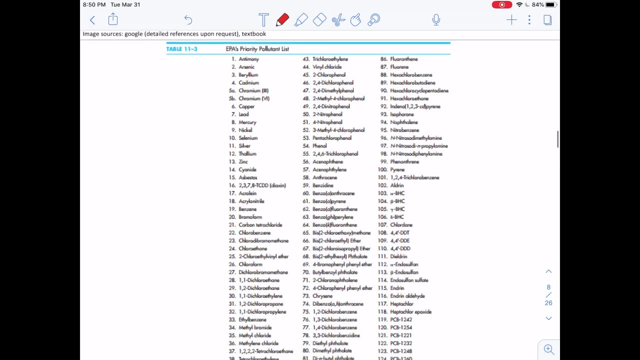 So you may say that, oh, the EPA is putting quite stringent standards in terms of the water quality, but look at this table here. So this is a table that's listing the EPA's priority pollutant list. okay, So this is all the. 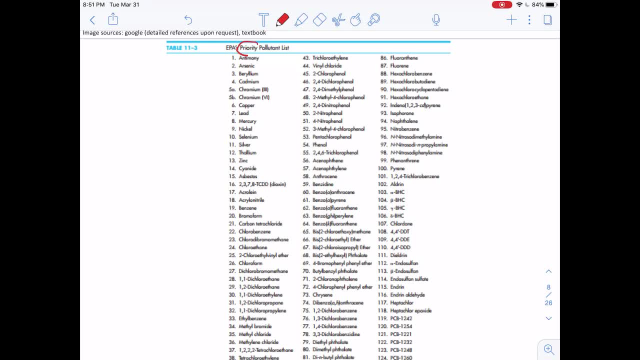 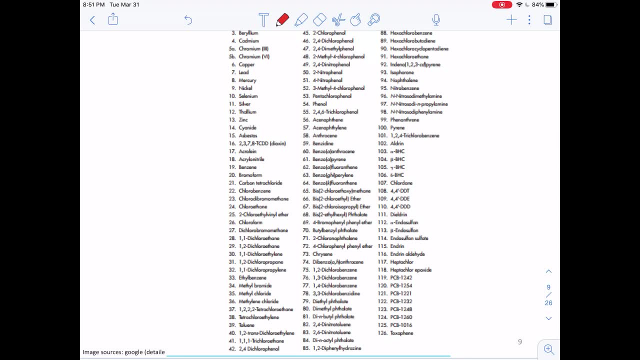 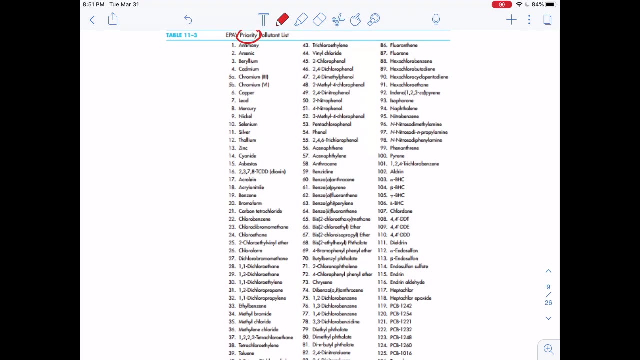 pollutants that the EPA is interested in, but also this is a priority list. you can see that in this list there are 126 different types of the pollutants, so if we really want to regulate the water quality in a more stringent standard, we need to measure the concentrations of all of these pollutants so that we can 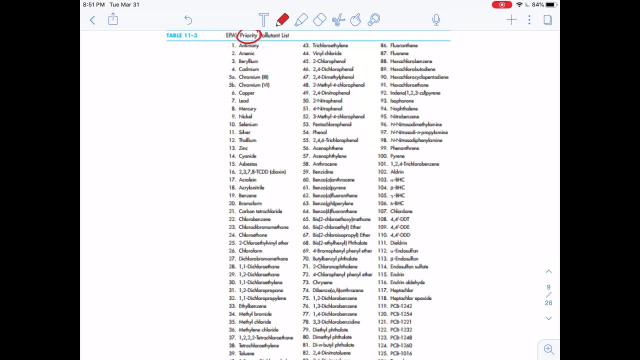 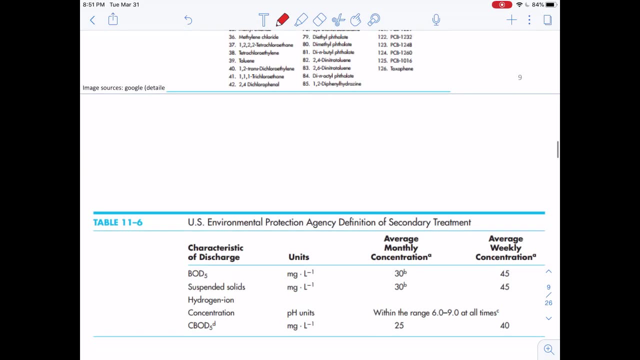 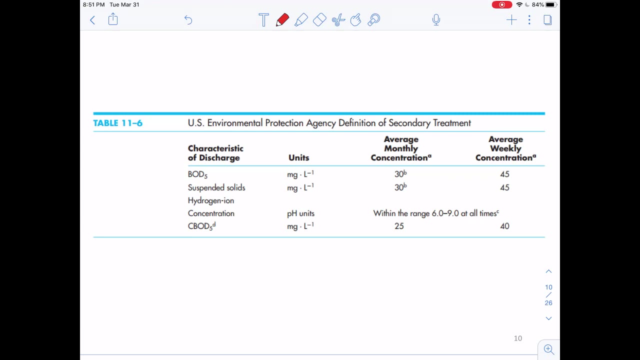 make sure that wastewater is safe to dump it back into the atmosphere, dump into the environment, or is even safe to drink. okay, so further. this is the limit that we'll talk about, or the standards the EPA put in regarding the concentrations of these pollutants. for example, for the BOD 5, it requires that 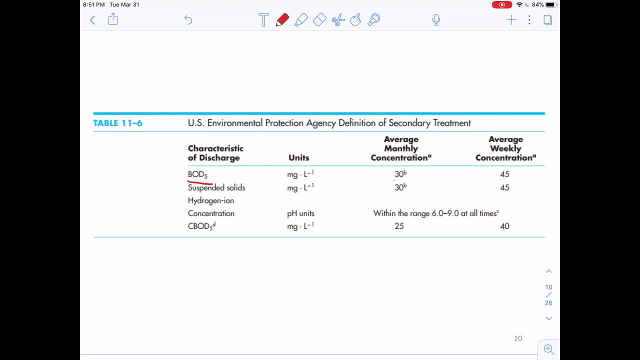 the monthly concentration, or the average monthly concentration, needs to be lower than 30, while the weekly concentration needs to be lower than 45. so, similarly, for these suspended solids we have, and the monthly concentration needs to be lower than 40 for the suspended solids we have. 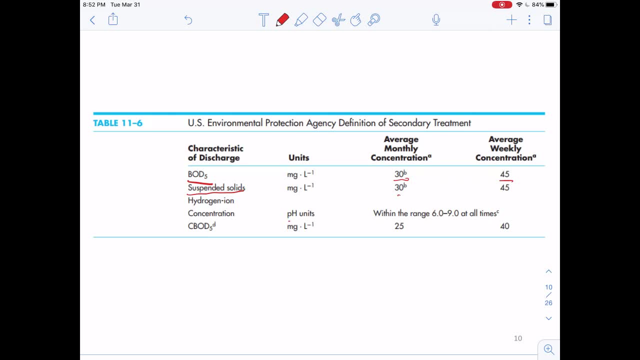 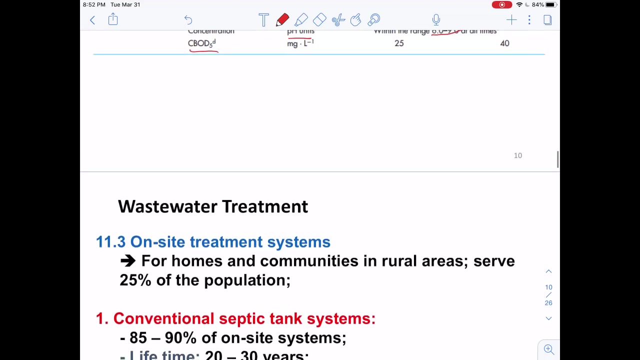 similar requirements. right, and in terms of the pH, it has to be in the range between 6 to 9, and for the CBOD or CBOD 5, it has to be in the range between 25 to 40. okay, so these are the requirements or the standards that people put on the 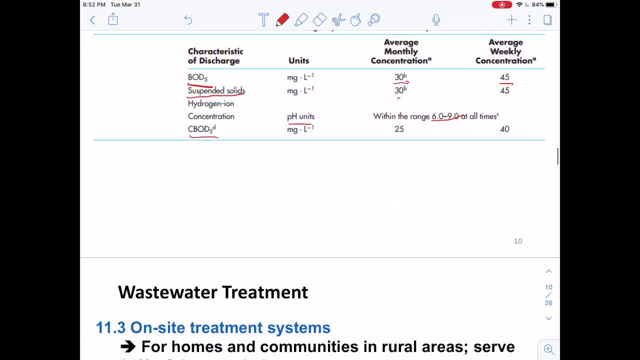 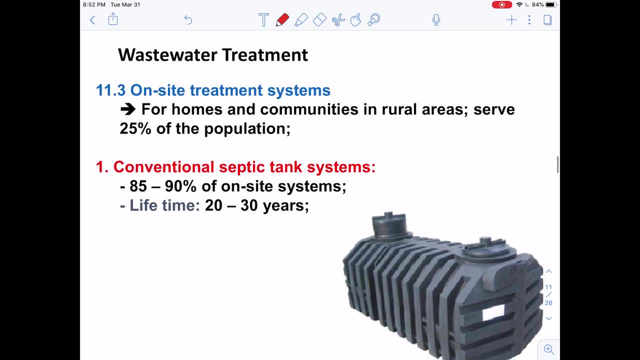 wastewater treatment processes. so now let's look into a few examples of the wastewater treatment devices. so the first system we're going to look into is the on-site treatment system. okay, so the on-site treatment system are different from the wastewater treatment plants, which are accommodating much more water. 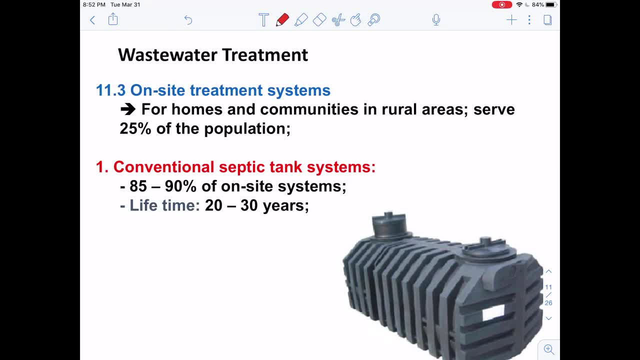 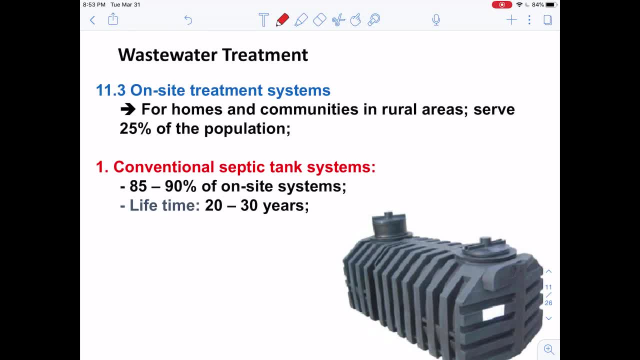 right, they can treat the water quality more efficiently. well, they can only accept a small quantity of water, so they're designed for homes and communities in rural areas and actually they serve quite a large fraction of the population. so they'll serve 25% of the population right and the rest of them. 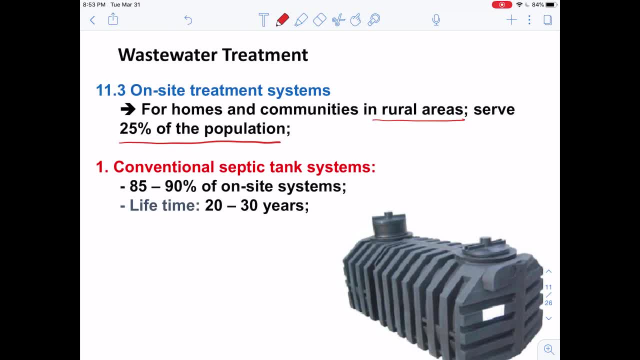 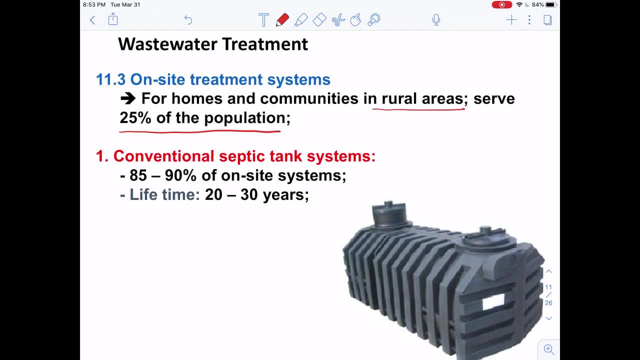 are actually served by the wastewater treatment plant. so the most important on-site treatment system is called the conventional septic tank systems. so as you can see later this, these septic tanks typically will have a quite simple structure there or quite simple mechanism there. so these conventional 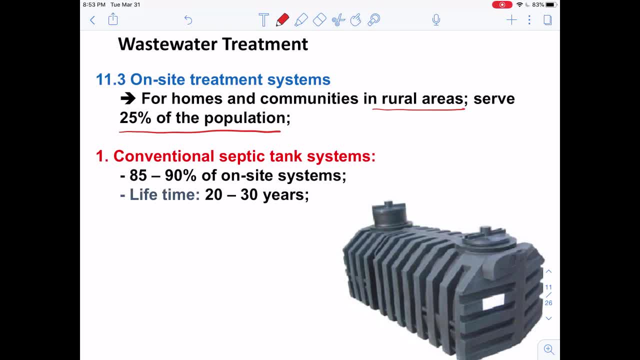 septic tank systems actually covers 85 to 90 percent of all the on-site systems and they also have a pretty long lifetime- from 20 to 30 years. but if you use for more than 30 years then you may have the leakage from the septic. 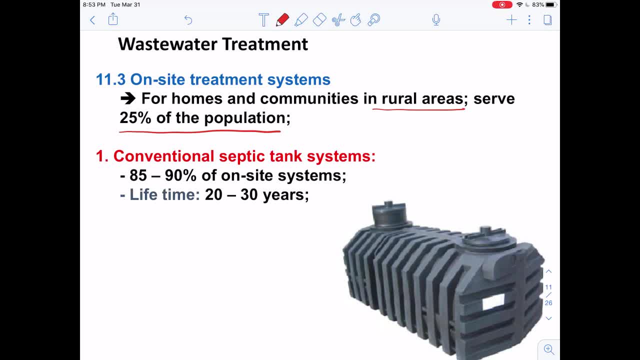 tanks and then these leaky septic tanks may come out of these septic water большой hotels. and then these leaky septic tanks may come out of these septic waterrays and then these leaky might cause pollution to the drinking water or the underground water and then further affect. 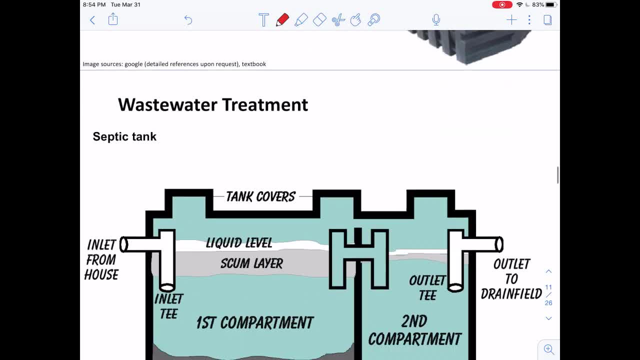 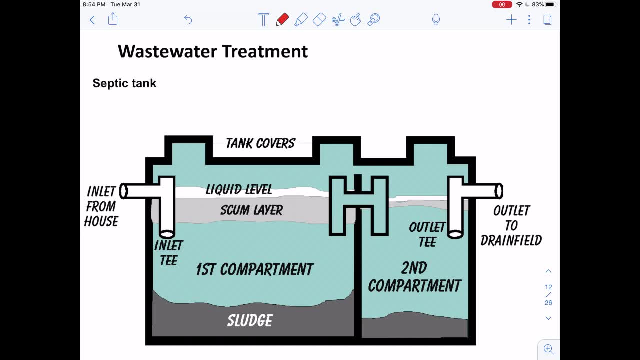 the drinking water's quality there. So, in terms of the mechanism of this septic tank- and here I'm just showing a very simple geometry here- So what happens is that the sewage or the wastewater coming from the house or coming from the community will be introduced into this inlet. 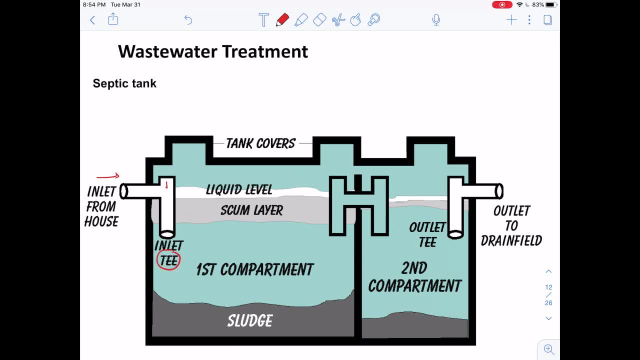 T here. okay, so the inlet T basically separates the gas from the liquid here, or liquid or solid. okay, so the liquid or solid will basically go to this first compartment, while the larger solids or the heavier particles are going to settle down, and we call these solids as the sludge, and then 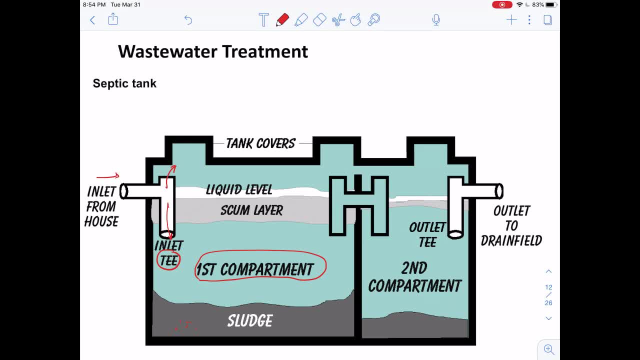 the liquid will basically exist above these solids here, and there are also is a layer called the scum layer, which is also quite hazardous, right, And we have a liquid level somewhere around here. okay, so then we have a piping system that's pushing this relatively cleaner, particle-free liquid into this second compartment. okay, because 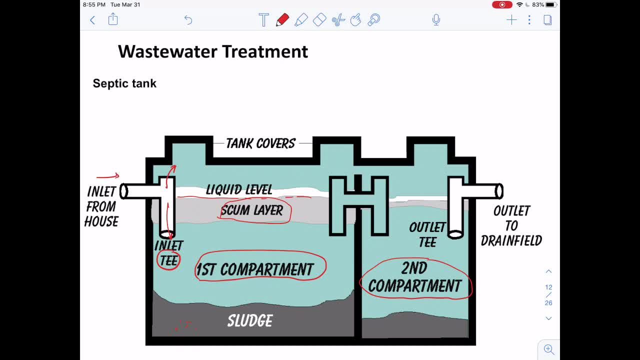 most of these solids are already moved and removed in the first compartment, so in the second compartment the remaining solids are going to take extra time so that they can settle down. We can also form these sludge here, but the water will eliminate the sludge, and form these sludge here, but the water will. 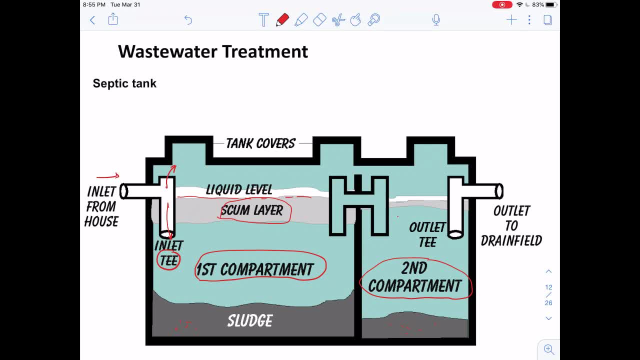 in the second compartment here are going to be more cleaner. so basically, we use this simple- let's say a baffled system to regulate the flow of the water and then we can get water that's with the treated quality. we're not saying that these water quality is good enough for drinking, but at least they're removed, or 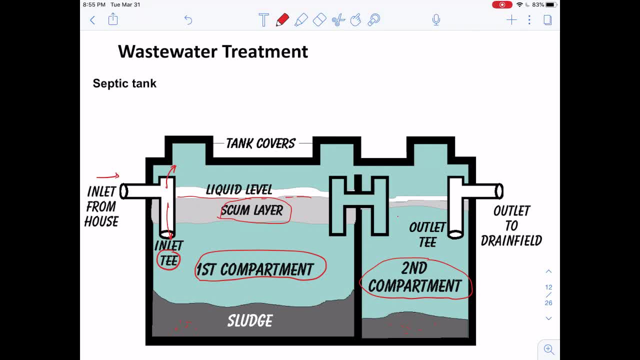 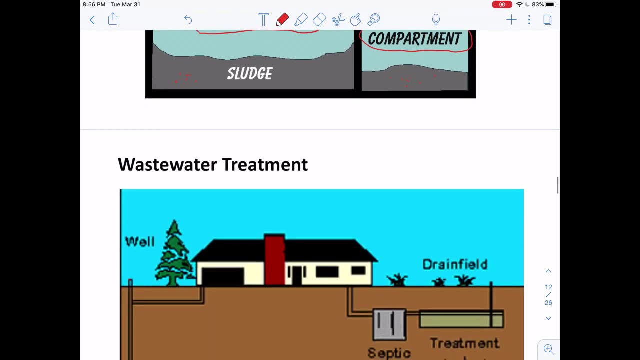 their concentrations of the contaminants, and especially for the solid particles, is much lower now. so then, after these water are being treated, they will be delivered from the outlet and then to a drain field. so here it is showing how the drain field works. so, basically, the wastewater is being treated by 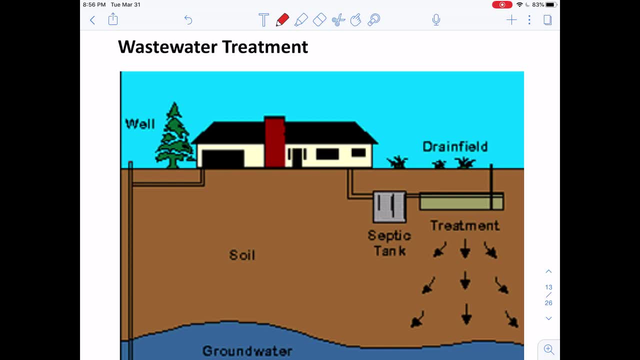 the septic tank and then these treated water will just go through these rocks or sand formations, right. so we know that the contaminants in the water, When they are in the solids or in the sands, there will be a retardation coefficient, So basically those contaminants will flow with a slower speed there. 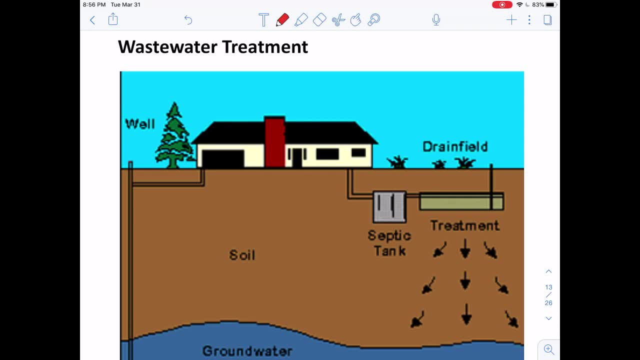 And also the speed here is very slow. We find that if two houses are separated by 100 meters- which is an example problem we talked about earlier- if they're separated by 100 meters, then it takes almost one year for the contaminant to move from the house A to house B. 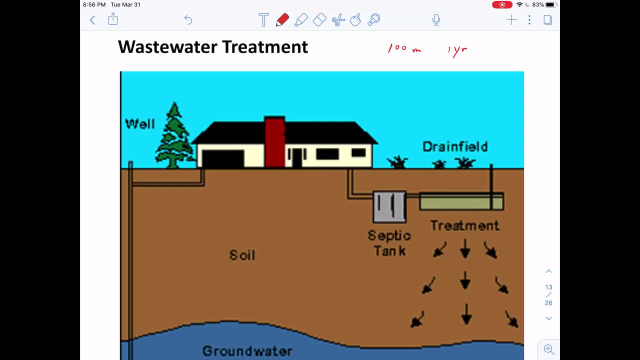 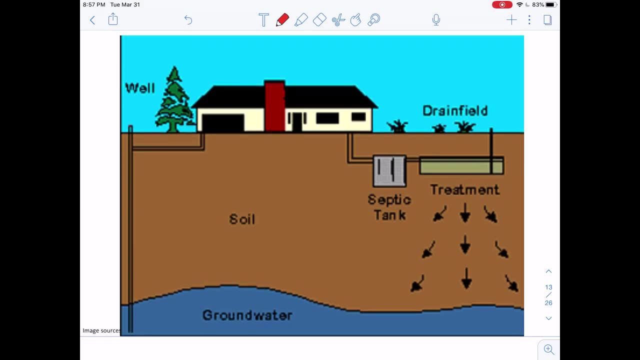 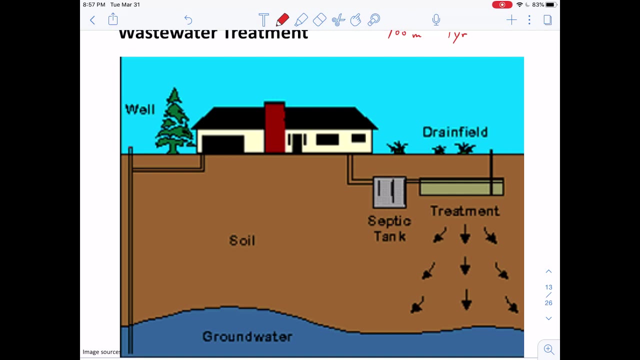 So basically, from these sand filtrations or rock formations here the water will get further purified and then the water can finally mix with the groundwater. But we're still quite concerned about the contamination of the groundwater source because we're using this groundwater as the 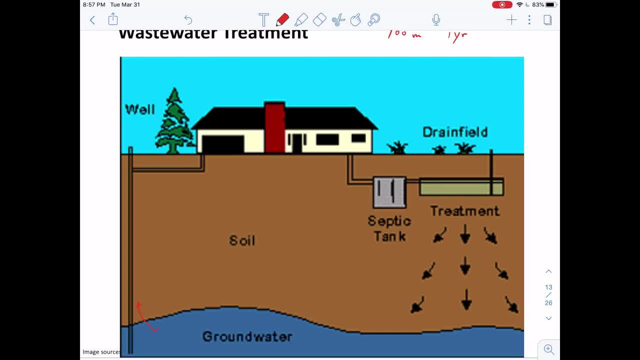 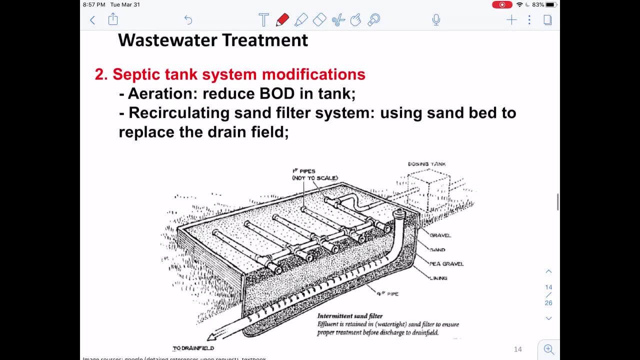 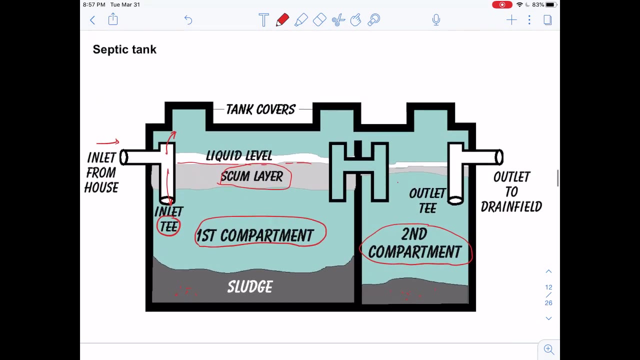 drinking water here, okay, So therefore we have to revise these septic tank systems right, So we can have the septic tank systems with modifications. So what we can do is that we can enhance the aeration. So if we enhance the aeration, what that means is we're going to introduce air in here. 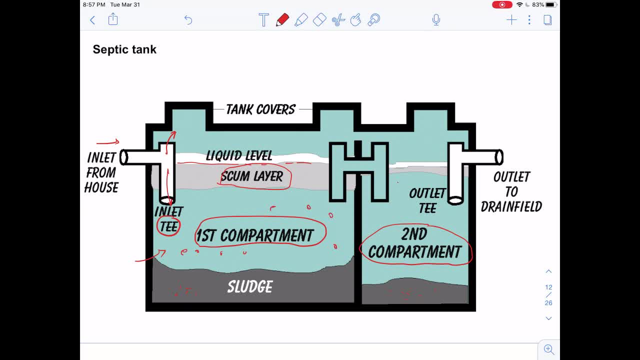 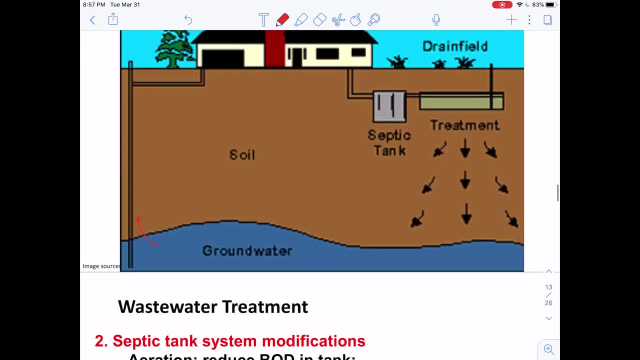 so generate a lot of bubbles here. So if we have enough oxygen, then the microorganisms in these wastewater are going to oxidize the organics or the organic components in the water so that we can remove or we can lower the BOD in the treated water, right, 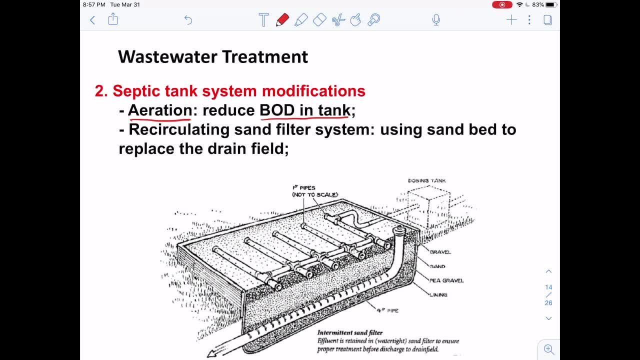 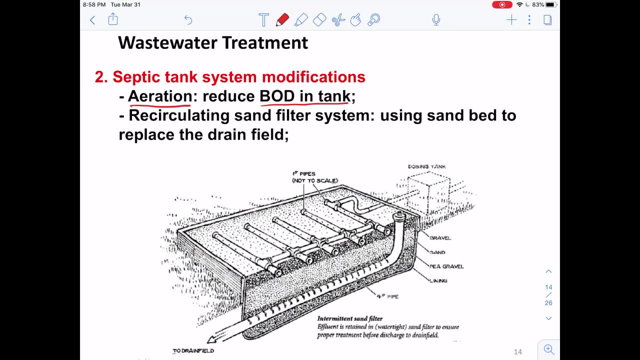 So we can reduce the BOD in the tank, And what we can also use is a system called the recirculating sand filter system. So this is quite similar to the idea compared to the drinking water system, the drink water treatment system, right. 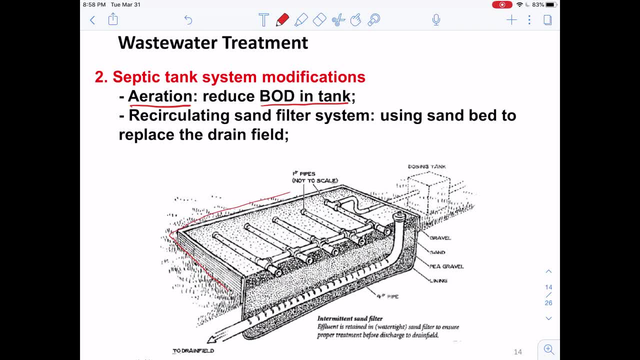 So basically, we have these sand filters here And then what we do is that after the water is being treated by the septic tank, it will be introduced into these pipes here, And the pipes have small pinholes right, So water are going to basically get emitted from these holes and then get filtered from these sand filters. 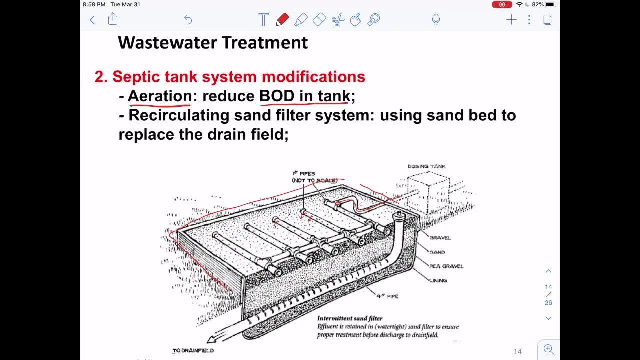 Okay, And then by this way we can remove the contaminants and basically leave them in the sand filters And then further we can collect them by these pipe here, And then further we can collect them by these pipe here, And then further we can collect them by these pipe here. 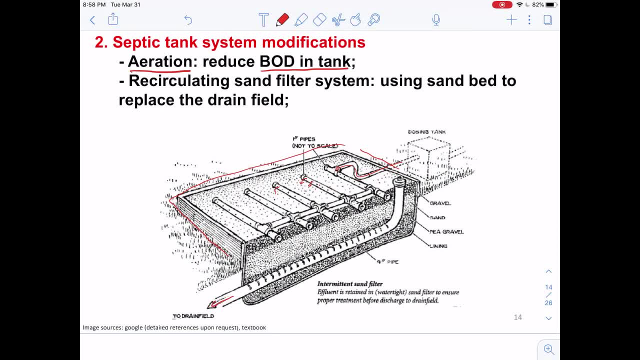 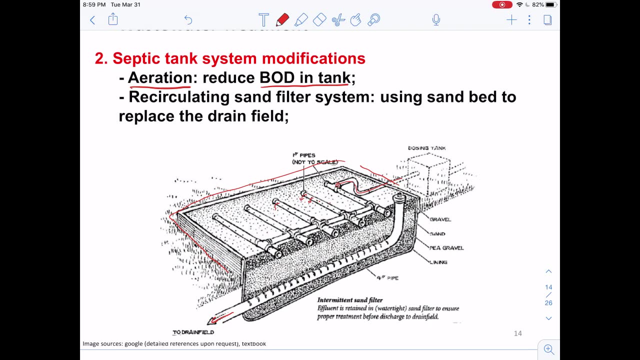 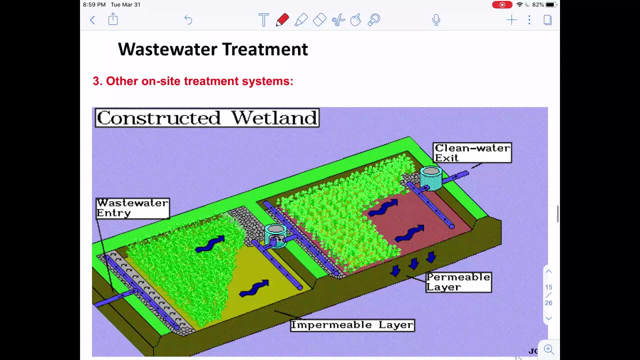 And then later introduce them into the drain field. So basically, this process: use the sand filtration to further remove the suspended solids and also some organic components or the chemicals from the water through the process called the adsorption. Okay, So there is another mechanism that's called the constructed wetland systems. 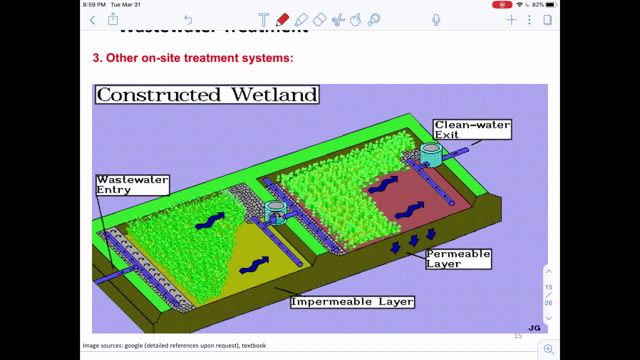 So what happens is that after the part, after the water is being treated by the septic tank, they'll be introduced into two compartments of the wetlands. So for the first part of the wetland they are composed of this impermeable layer. 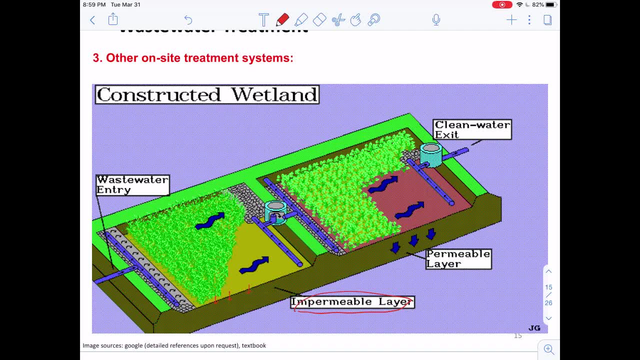 So what happens is the water is not going to get transported further lower down there, So the only way the water can flow is horizontally through the wetland. Okay, So in this way the water can get filtered And then at the same time, 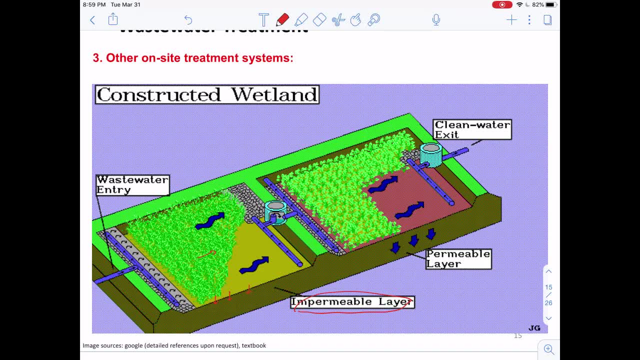 while they are being filtered, they leave those organics or the nitrogen phosphorus in the soil or in the sand, And then these are the nutrients for the plants or for the organisms that's living on this wetland. Okay, So then, after the water is being filtered, 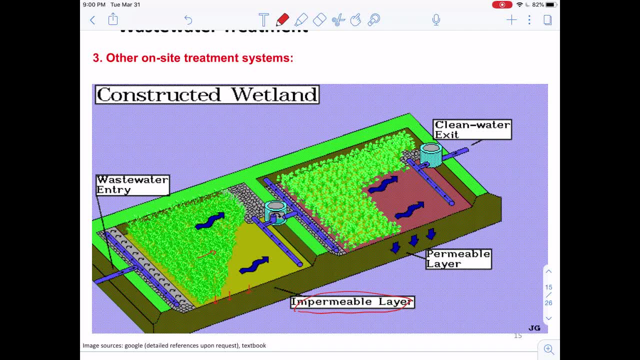 they will be introduced into the second part of the wetland And further for this part of the wetland they will have the permeable layer Where the water can further diffuse or settle down into further the groundwater. But still we're able to collect some of the water from the second part of the wetland. 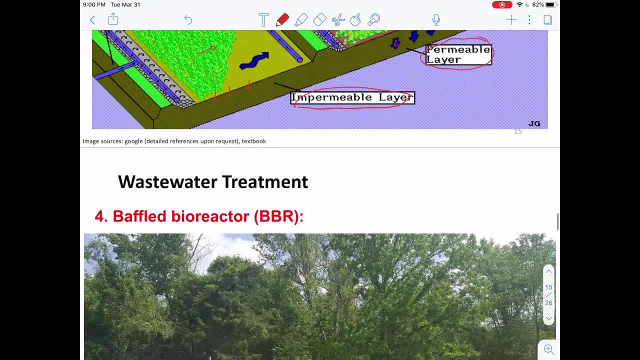 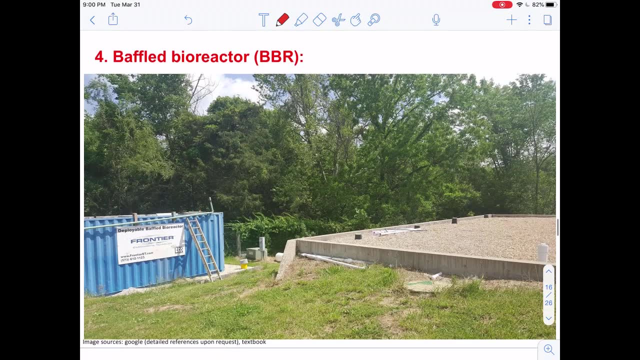 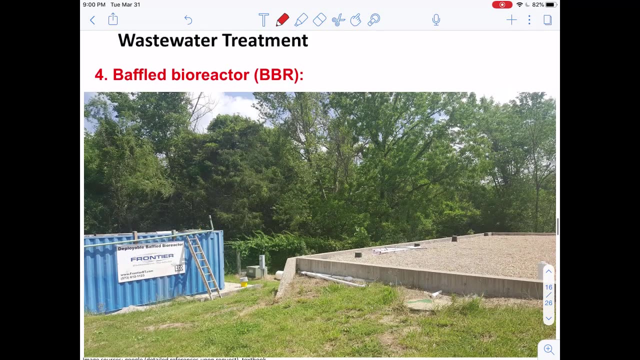 And then they can exit from here. Okay, So, apart from these systems, there's also a system called the baffled bioreactor system or the BBR. This is also quite widely used, especially for the military use, Because in military, when they move to different locations, 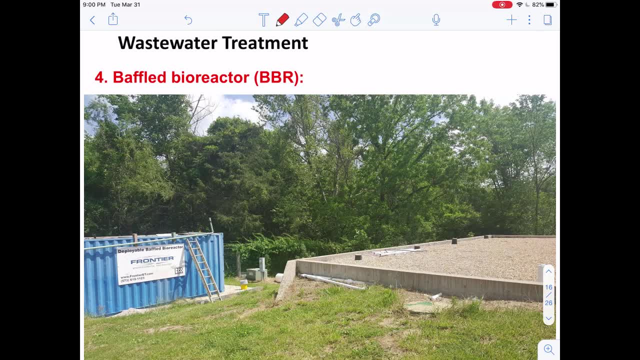 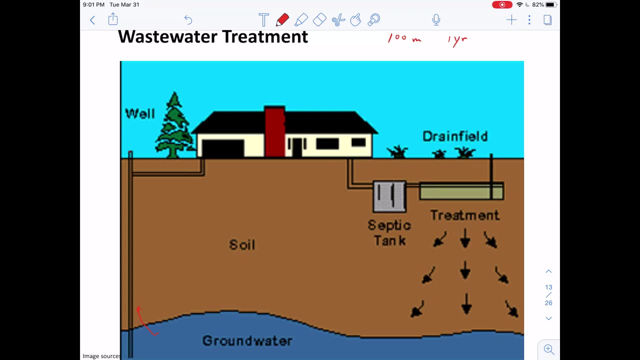 they want to avoid the contamination of their drinking water source from the wastewater right. So you have to make a very condensed system where it can sit just above the ground, Because if you look at the septic tank, they typically exist pretty below the below the land surface. 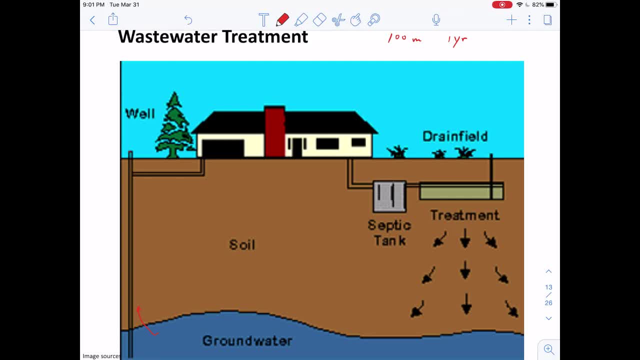 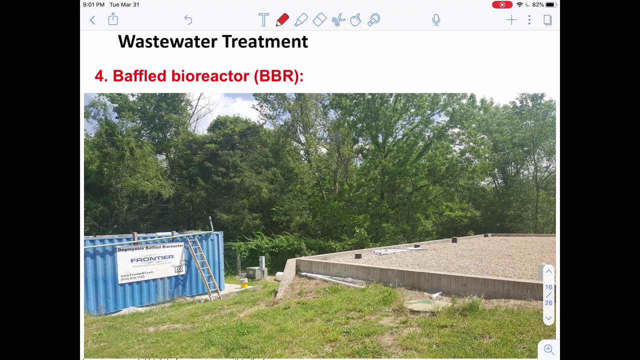 right, Because water have to use density, They have to use this gravity to go into these tanks here. But for these baffled bioreactors they can just sit outside and then just above the ground And then it is also a pretty condensed system where you can treat the water quality quite efficiently. 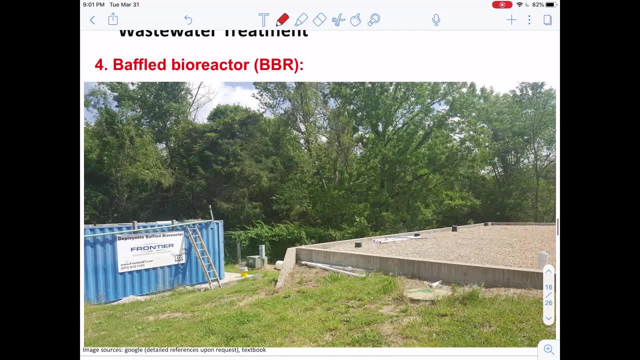 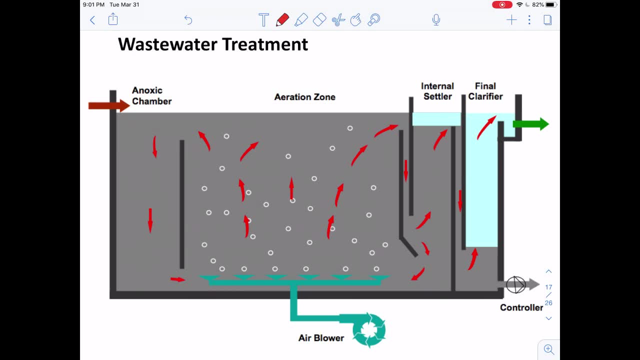 So what happens in this baffled bioreactor here is that we'll introduce the wastewater first by through this anoxic chamber. Okay, So what happens in the anoxic chamber is that we're achieving the denitrification, which is converting the nitrate into ammonia or the ammonium ions. 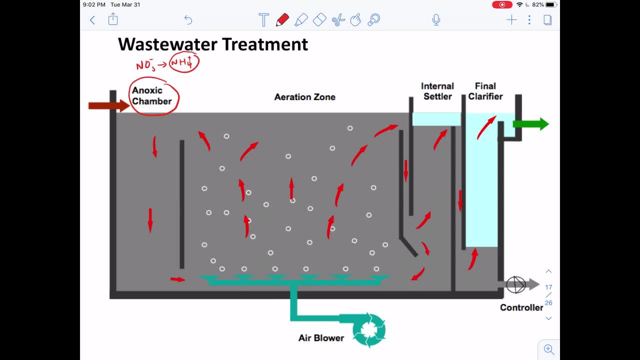 Okay, So by doing this we can further enhance the oxidation process of these nitrogen species. Okay, So, basically, after they are being treated, they will be introduced into this aeration zone here. So inside the aeration zone, we're bubbling oxygen or air in the water. 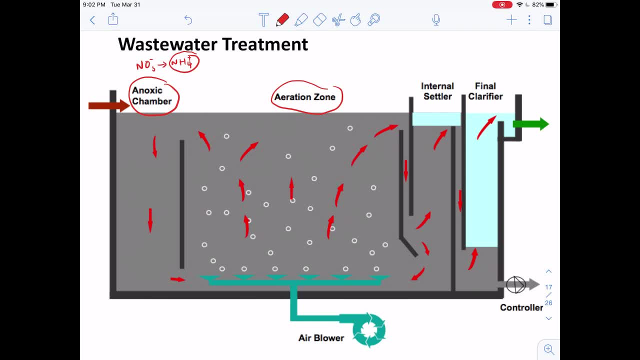 So this is, on one hand, is oxidizing the organics in the water right. On the other hand, is also oxidizing these ammonium in the water. So at the same time, the larger particles are going to settle down to the base. 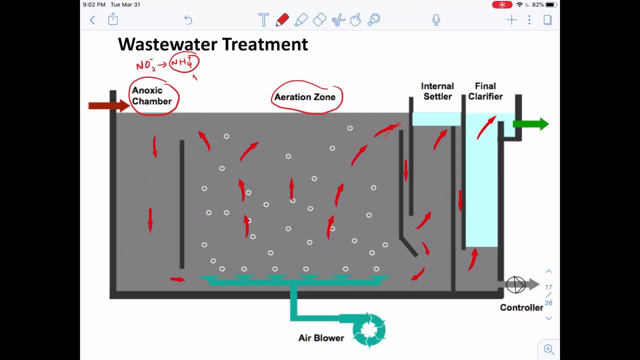 and then we're going to obtain relatively cleaner water from the top here And then by these baffles or channels here they'll further flow by, So to give them a longer residence time, so that particles can settle down, and then we're able to basically get cleaner water from these different channels. 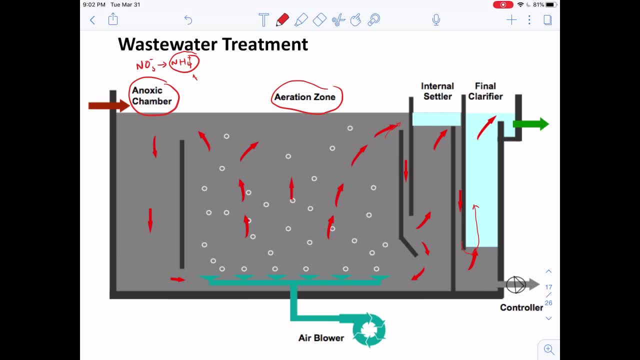 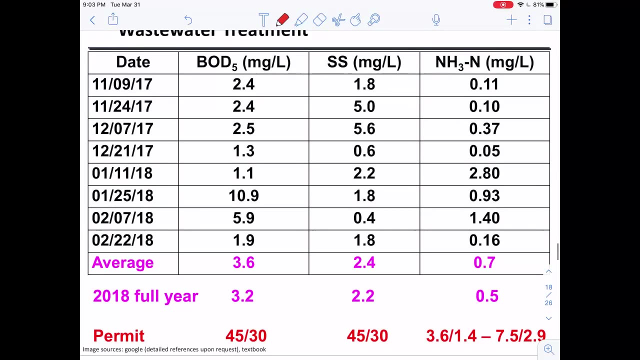 So you can see that it needs a relatively longer residence time in order to remove these contaminants from the water, right? So in this way we can also treat the water quality. So how do we make sure That the water quality is good enough? 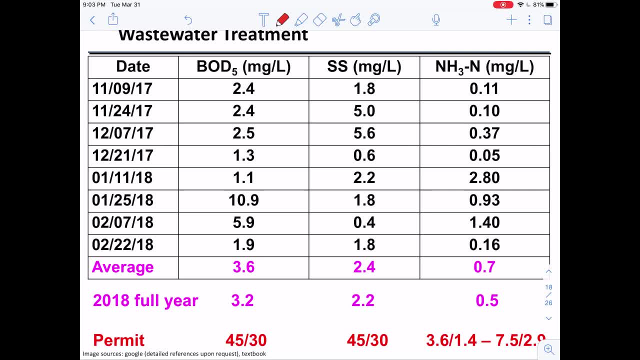 right. How do we make sure that it satisfies the standards established by the EPA? So what we do is that we'll typically measure the water quality or the, for example, the BOD5 suspended solids and nitrogen every after some time. Okay, 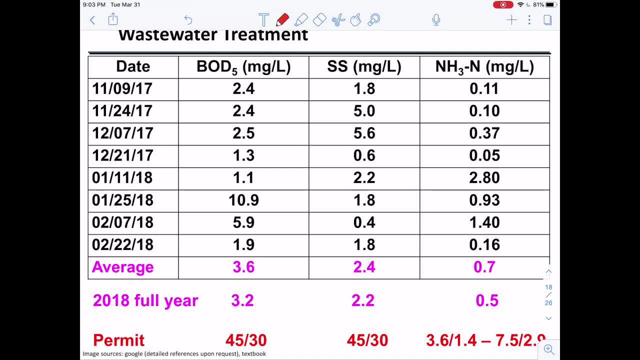 for example, this is measuring the wastewater quality for every two weeks. So you can see that there is indeed some fluctuations, because it really depends on what are the, what are the supplies and demand right, Maybe for some time, for some time period? 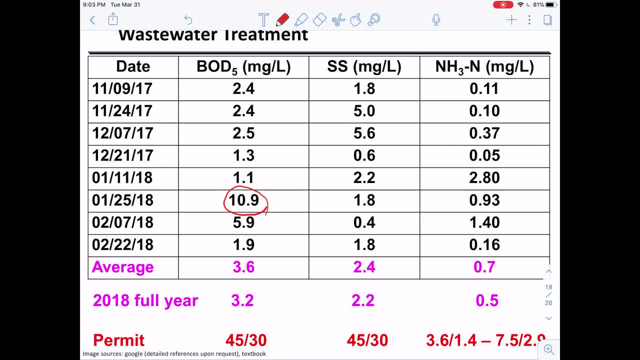 there is more emission, or there's some activities going on in the industry or at someone's home, so that the water coming from that event is more polluted. Okay, but if we take the average of all of these constituents and try to find out what are the average values? 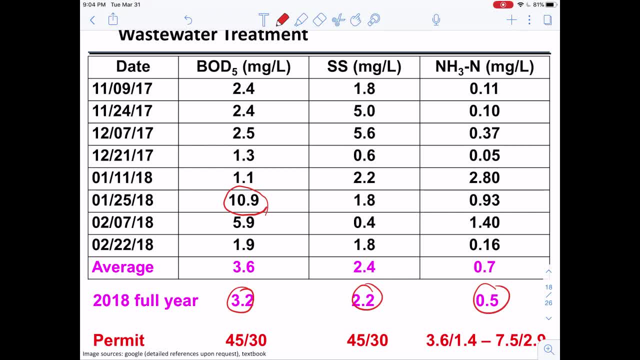 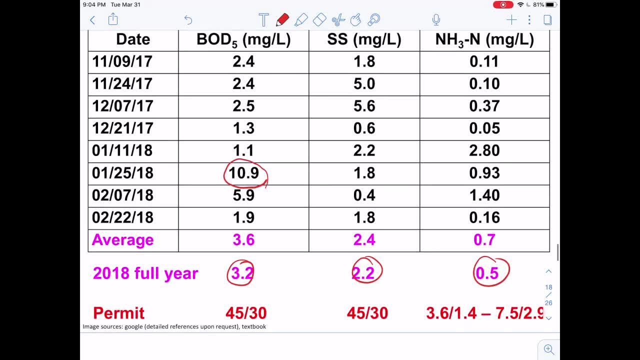 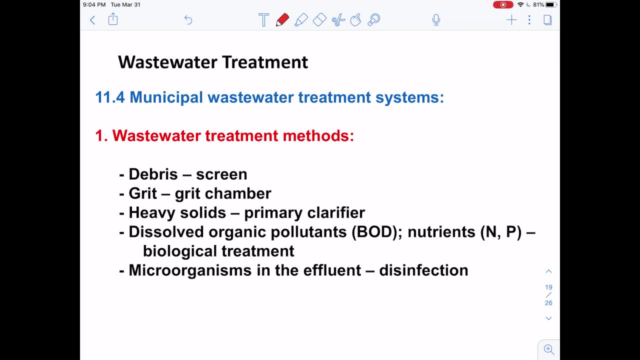 then we can compare that against the EPA standard. there You can further tell whether they satisfy the requirements or not. Okay, so this is all about the on-site wastewater treatment systems. So there are larger scales of the wastewater treatment plants, which is the municipal wastewater treatment systems. 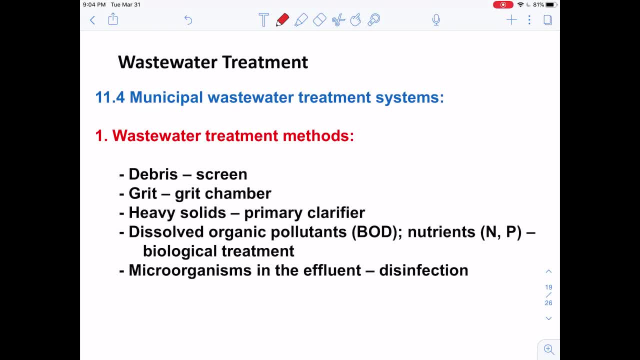 Okay, so they will be composed of more detailed procedures. For example, we have to remove the large debris by the screening method. We have to remove the grit, which is basically the larger particles, by a device called the grit chamber And, as you can see from the video, 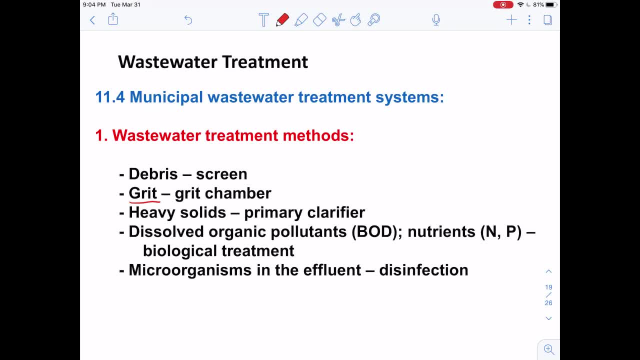 there are three different types of the grit chambers And for the heavier solids, we'll use the primary clarifier to remove these particles. In terms of the dissolved organic pollutants, or the BOD, or the nutrients, we're going to use the biological treatment. 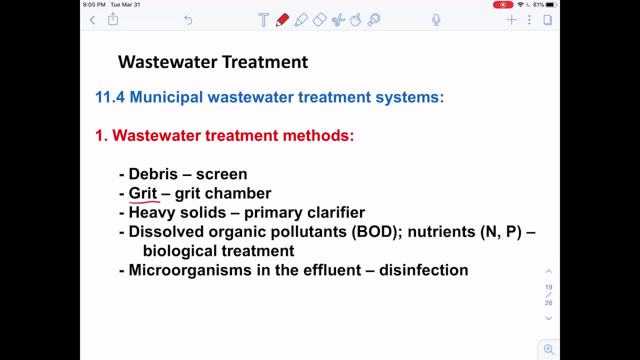 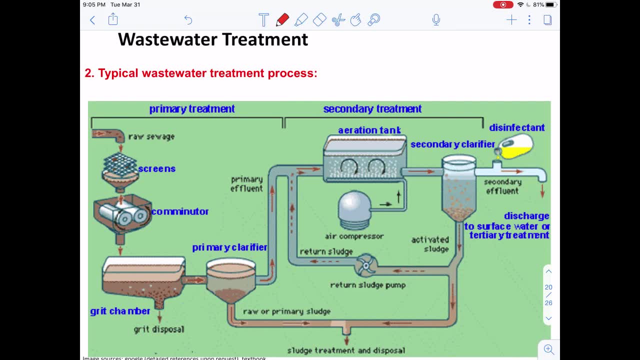 Okay, and for the microorganisms in the effluent we'll use the disinfection. So here we're going to go through the treatment process, which is similar to the contents shown in the video here, but it's shown in this graph here. 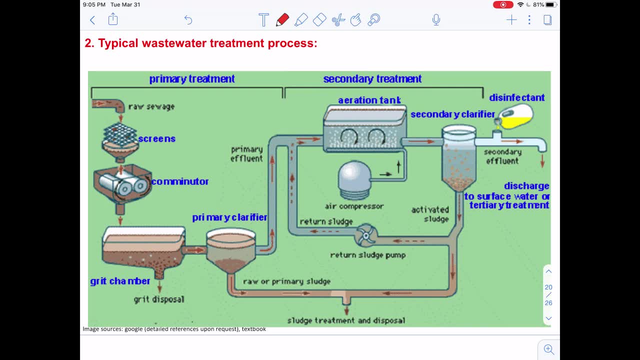 So after the wastewater being collected, we call them as raw sewage, So they will go through the screens, Okay, or the bars right to remove these larger debris or larger chunks of the solids. So here is showing a new, new device that's called the comminuter. 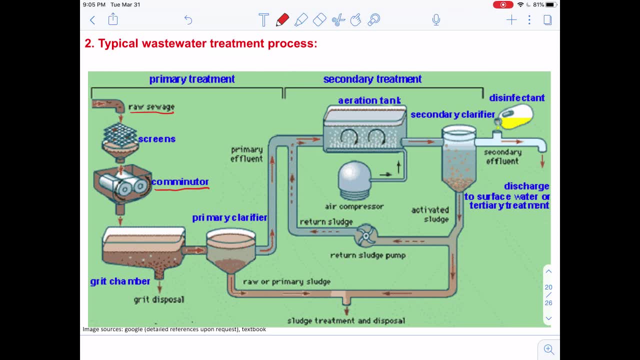 right. What the comminuter does is basically break down the larger particles into small pieces. Okay, but I don't think in our textbook we covered this device here. So basically it's converting these larger particles or curing these larger particles into smaller suspended particles or the grits. 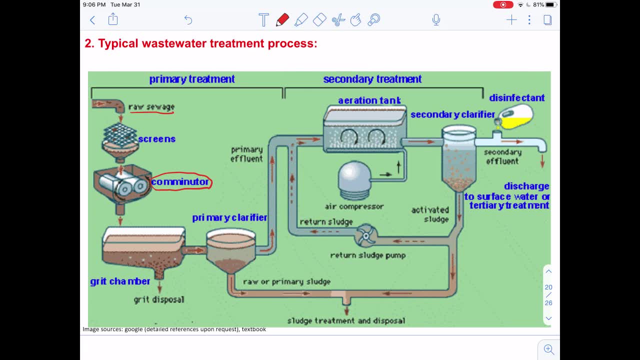 Okay, so then the water will be introduced into this grid Chamber where these larger particles are going to get removed, and then they will go into- they're going to introduce into the primary clarifier, right? So the particles will further settle down. 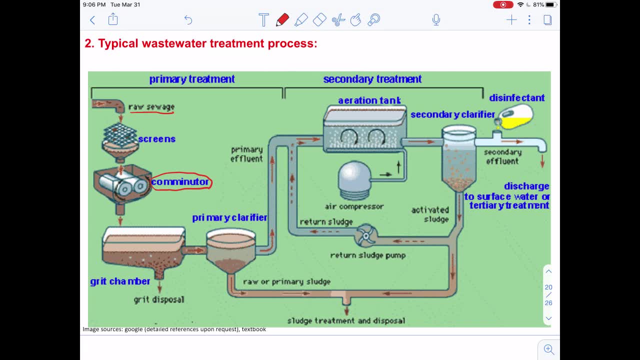 right, And then the cleaner water will go to an aeration tank. So inside the aeration tank we're bubbling a lot of air right. to maximize the oxidation of the organic organic components in the water. to lower the BOD values. 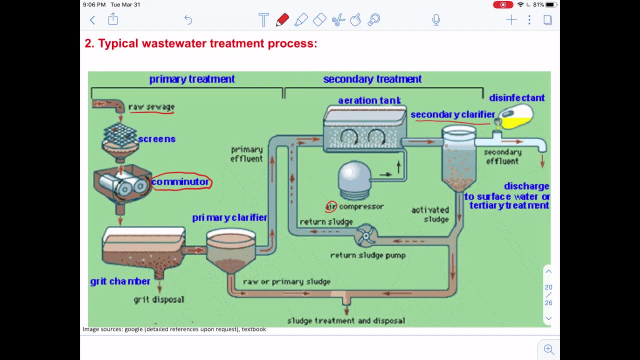 So after we get these cleaner water, they will go to this secondary clarifier and inside the secondary clarifier, what settles down- here we need to pay attention- will be largely composed of the microorganisms. right, We need these microorganisms to maximize the oxidation process in this aeration tank. 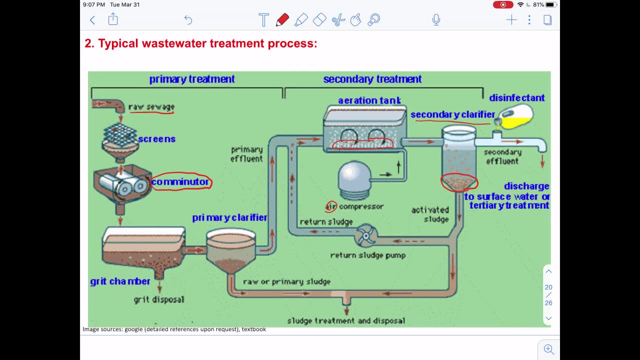 So that's why we also call this constituents as the activated sludge, And what we do, what we do, is that we will take a part of these activated sludge back into the aeration tank right. So, as the video shows, 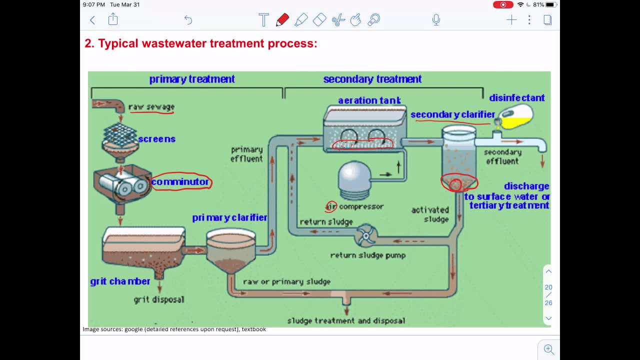 so these are basically the microorganisms or bacteria that can eat unlimited food right, So they are always consuming these organics in the water by using these recirculation process here. So after we get these further cleaner water, we can use the disinfection to remove the microorganisms. 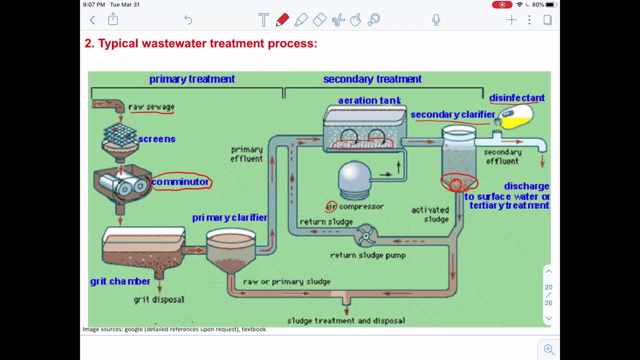 We can either discharge them or send them to a tertiary treatment, right? So one thing we need to note is that. so here, although we are separating this entire process as a primary treatment and secondary treatment, but inside the primary treatment, people will also categorize these three processes as the. 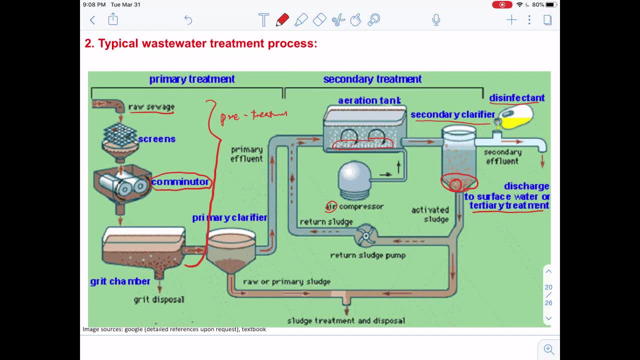 pre-treatment. So this really depends on the definition of the treatment processes. According to our textbook, these processes are called the pre-treatment, while the primary treatment is just this primary clarifier here, while the secondary treatment will include these aeration tank. 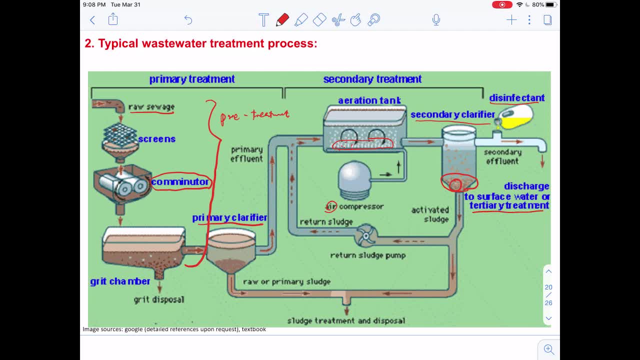 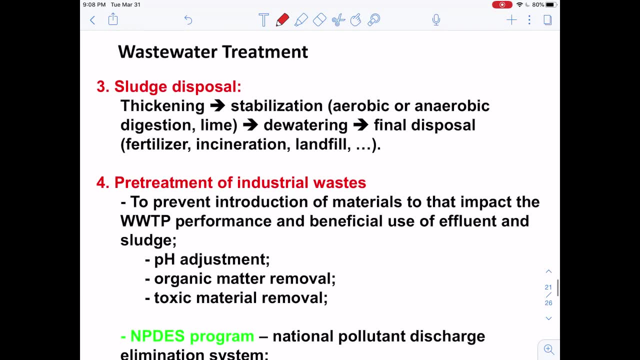 secondary clarifier and also these activated sludge process. Okay, So, as you can see from these processes, one thing that's quite different from the drinking water system is that we need to involve this sludge disposal right. So the wastewater contains a lot of solids inside the wastewater. 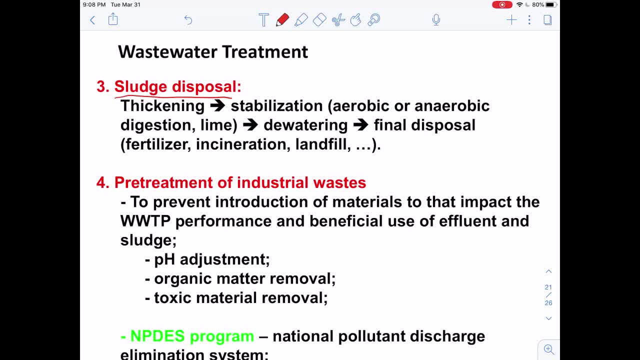 right. So we have to remove these sludge from the wastewater. So a serious process is being used to dispose these sludge. So we have to first thicken the sludge here, which is basically to make it more, more condensed or concentrated. 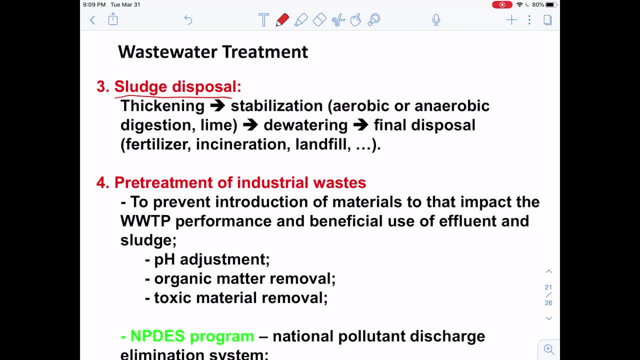 And then we need to go through the stabilization, dewatering, and finally it's a final disposal. Okay, so they can be used as fertilizers, or they can just go to the incinerators to go through the combustion, or they can just go to the landfill. 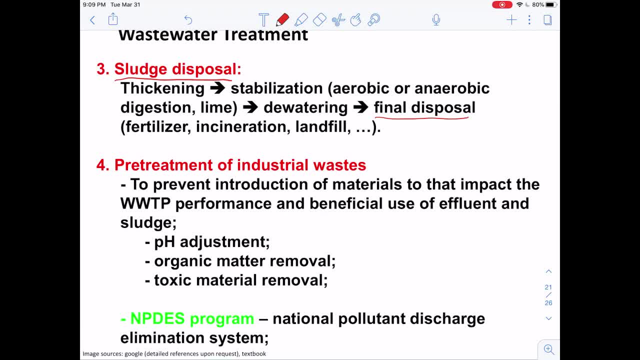 And in terms of the pre-treatment of the industrial waters. again, this really depends on the definition of different treatment processes. So the wastewater treatment plant will also adjust the pH or remove some of the organic matter or the toxic material removal.